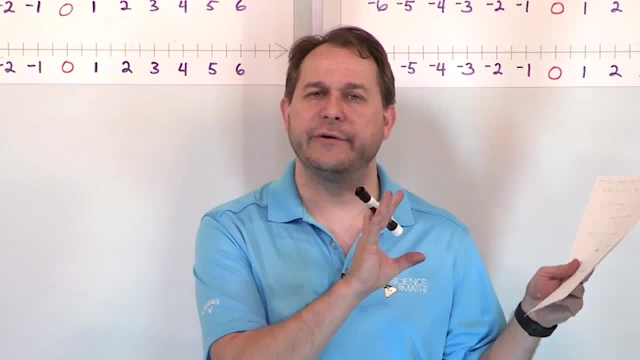 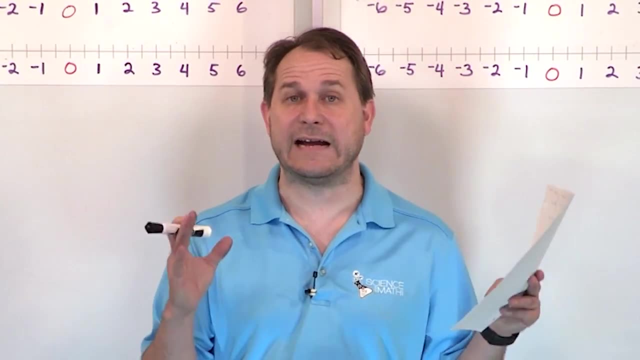 so that you don't have any problems here. The basic idea is: first what we're going to do is review what absolute value is, and then we'll show how we can write an inequality that also has an absolute value signs in there and how to handle it. So the first 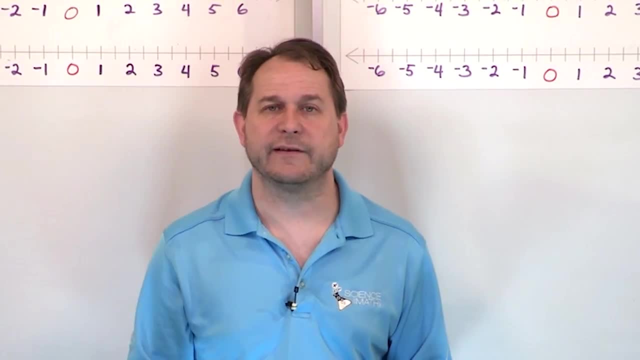 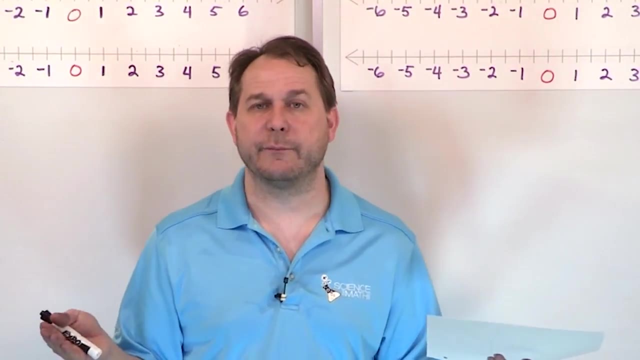 thing I want you to remember. I guess there's one thing I want you to remember in the back of your mind as we do this lesson: Absolute value means how far away that number is, or how far away the number is from zero, how many units away it is from zero In other 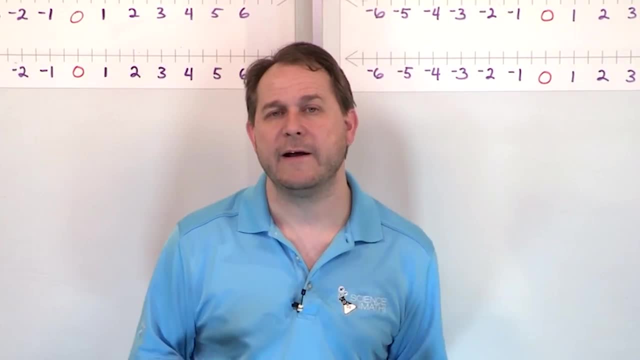 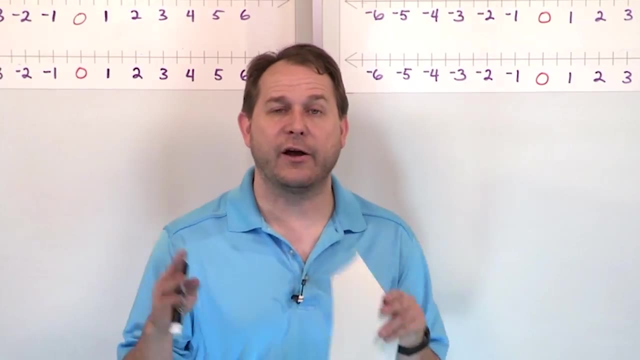 words. absolute value means distance from zero. That's what it means. I know you all know that absolute value of three is three and the absolute value of negative three is also three. But what that means is the negative three is three units away from zero. that's its. 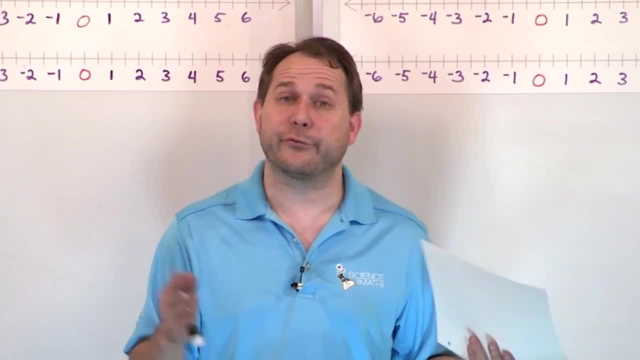 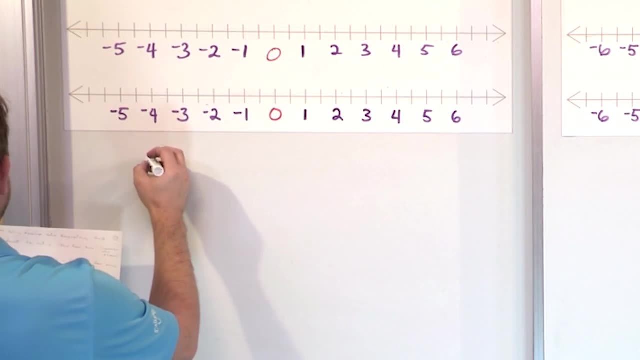 absolute value, and the absolute value of a positive three is also three units away from zero. So I want you to keep that in the back of your mind, because it will help you when we solve these problems. So let's take three cases of very simple absolute value. 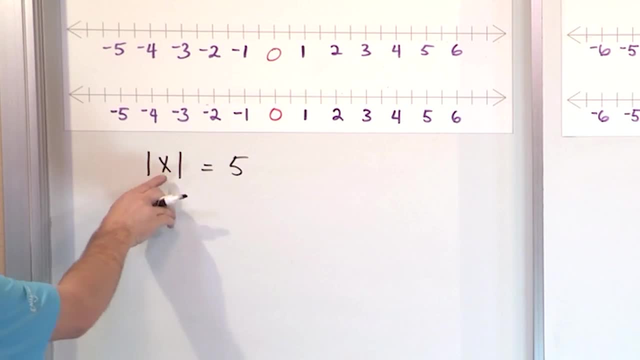 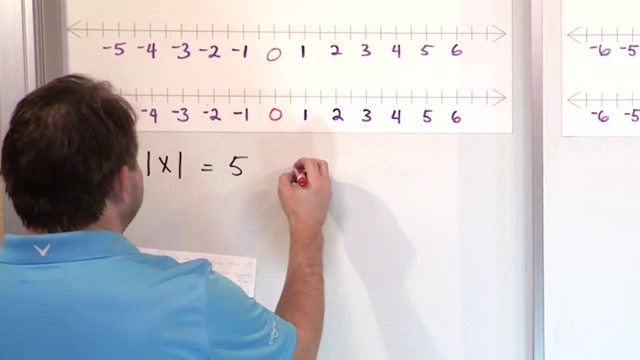 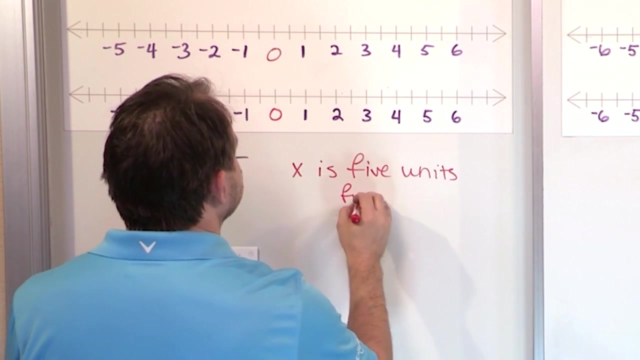 kind of deals. If we say the absolute value of some variable, x, is equal to five, what does it mean? It means that whatever is inside of there, it means that x is equal to zero. It means that x is five units from zero. It means that whatever x is, once I take its. 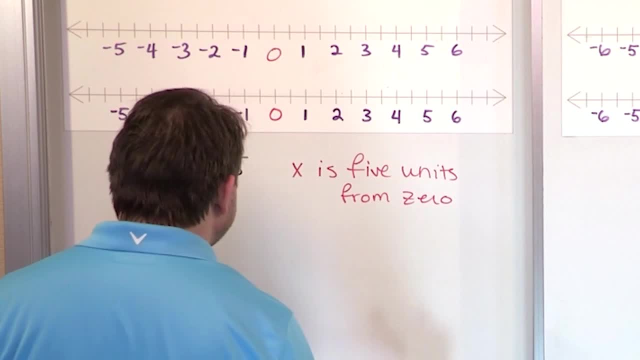 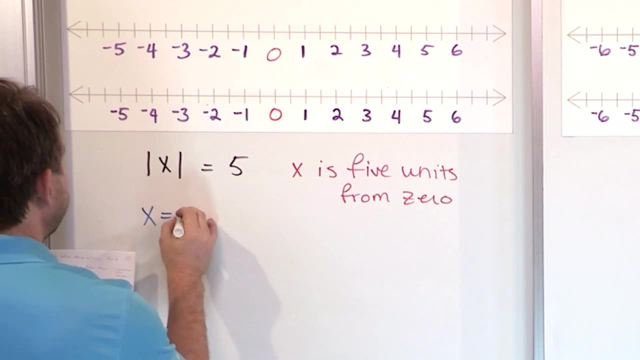 absolute value, it's five units away from zero, So there's only two numbers that make sense for that. for this particular example- And we all know that- this means that x can be five because we put the five in there- the absolute value is five or x can also. 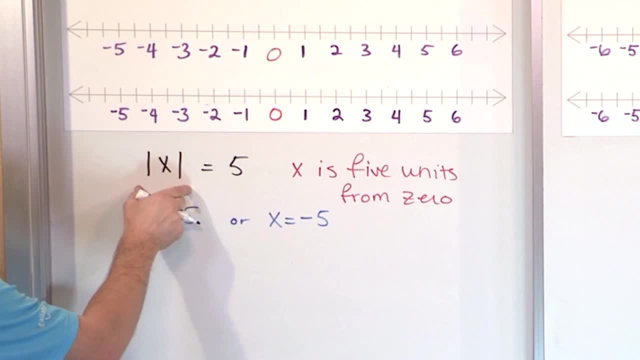 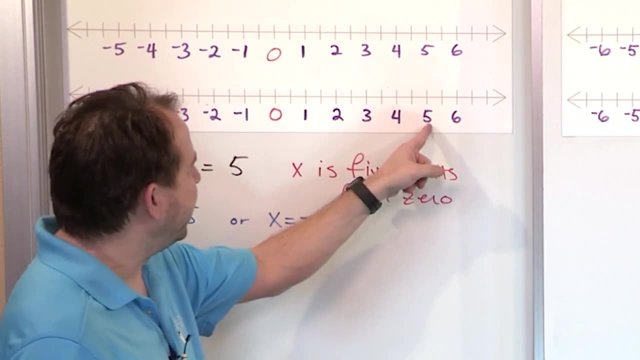 be equal to negative five, Because if we stick negative five in there, it means that x is five in here, and take its absolute value, we also get five. So another way to rephrase everything that we have on the board is that the number five over here is five distance. 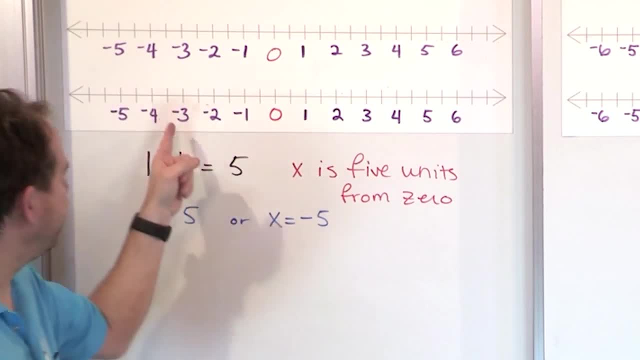 units away from zero and the number negative five, which is over here, is also five distance units away from zero. So if we were going to plot this, if we were going to plot the answer to this, this is not an inequality, this is an equation. The two solutions of 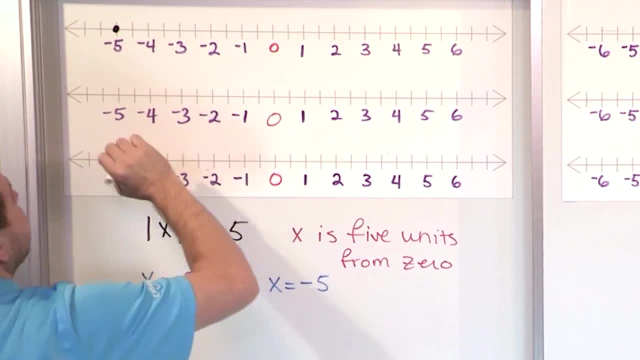 five and negative five would be what, It'd be a dot over here at negative five and it'd be a dot over here at positive five. Right, And these, this is the only two points that satisfy this equation, because we put one of them in here, we get five. We'll put the other one in here, we also get five. But 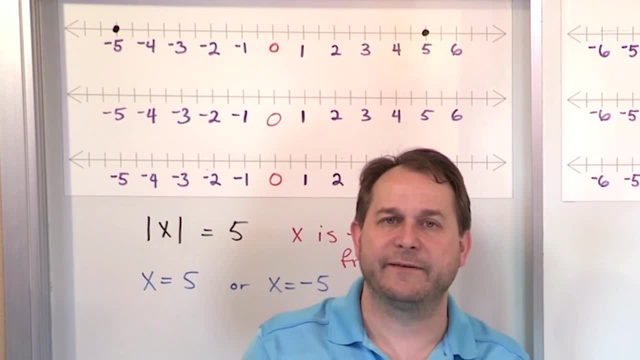 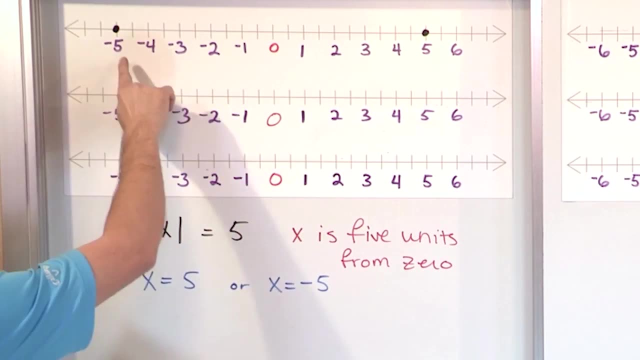 more fundamentally, I want you to remember that when you see an absolute value, it means that whatever's on the inside is five units away from zero. Five units away from zero is what this one is. five units away from zero is what this one is The reason I want. 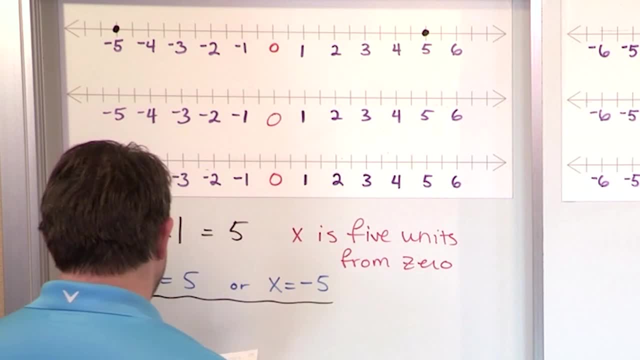 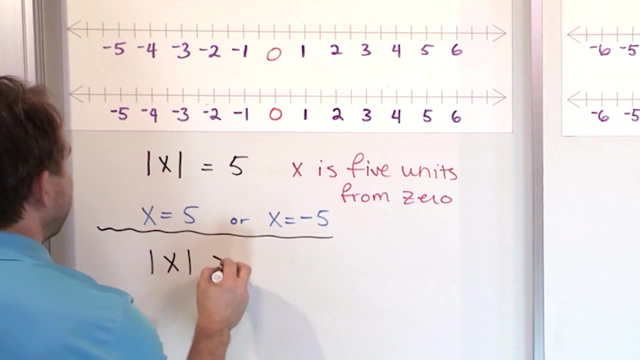 that to be in the back of your head is because it will help you when we discuss the next part. Let's say we had another guy, but this is not an equation anymore. it's a very simple inequality that involves absolute value. Let's say, the absolute value of x is greater than. 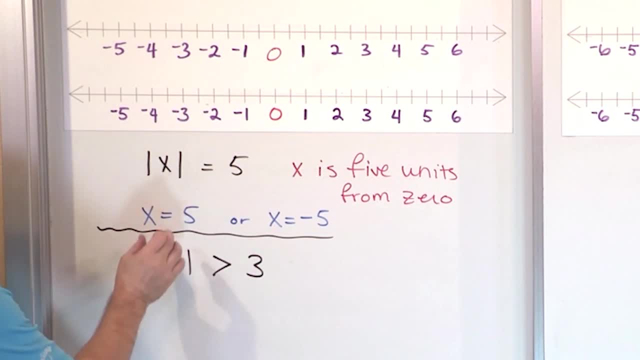 three. What does this mean? It means that now we're not going to be getting just two points back, we're going to be getting a range of values or multiple, just like we're always doing, all these absolute value problems. we always get shaded areas on the number line. 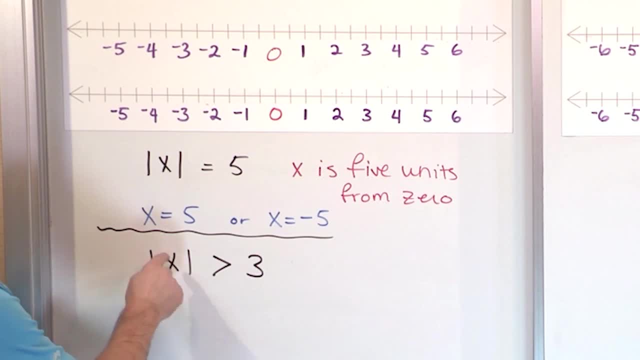 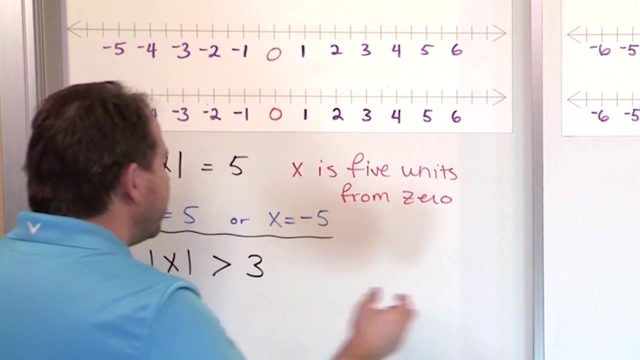 But what we're saying is, whatever the answers for x are, the absolute value of them will be lower, but x and x, and x coming from zero must be greater than three. So the set of numbers is what we're saying. x is going to be has got to be three units or more greater. 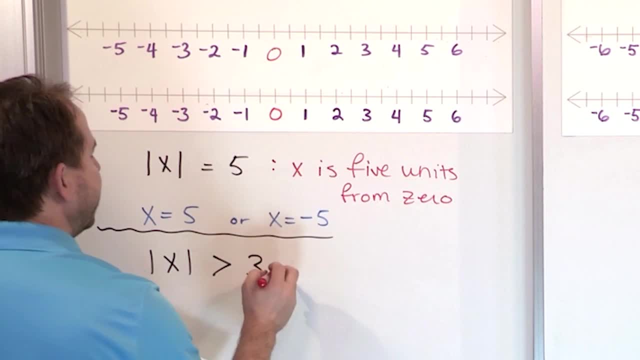 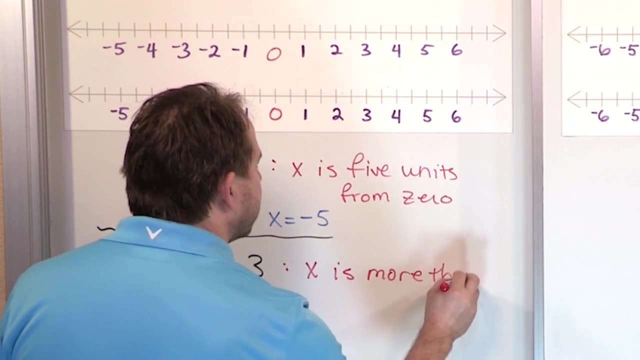 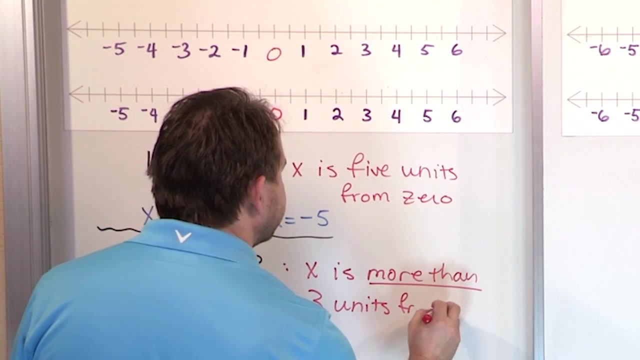 from zero, bigger from zero. So let me write that out real quick. So what this basically means for each of these we're going to write a couple of cases here. we say x is more than more than three units from 0.. 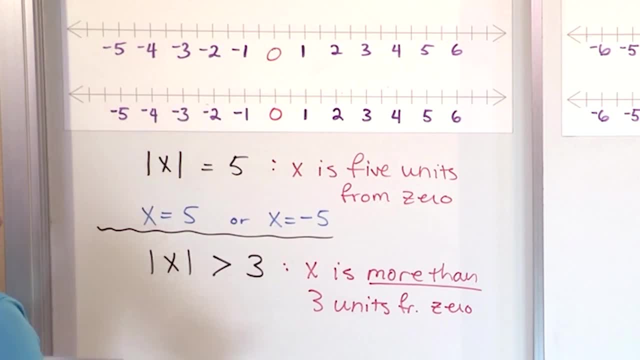 So when you rephrase it in terms of English like that, then it's a lot easier to find out what the answer is. When we say it's more than three units from 0, what we're saying is that X has got to be greater than 3. that would be three. 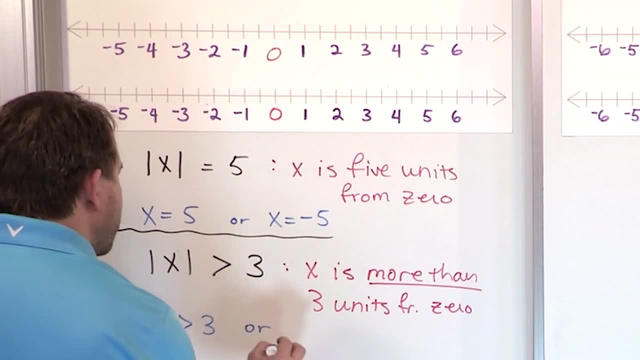 units away from 0 or more, or X can be- this is the part where you gotta start paying attention- less than negative 3. Either one of these means that the set of values of X will be bigger than three units away from 0, and let's to see why this is the case. let's plot both of 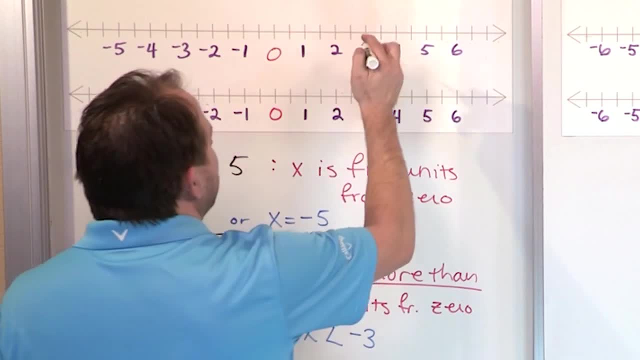 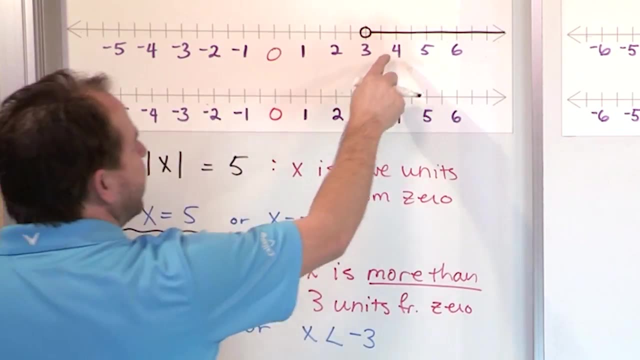 these on the number line. What is X greater than 3?? Well, X greater than 3 would be open circle at 3 and it would be all the values to the right of this. X greater than 3 would be 4,, 5,, 6,, 7,, 8 and all the little decimals in between. 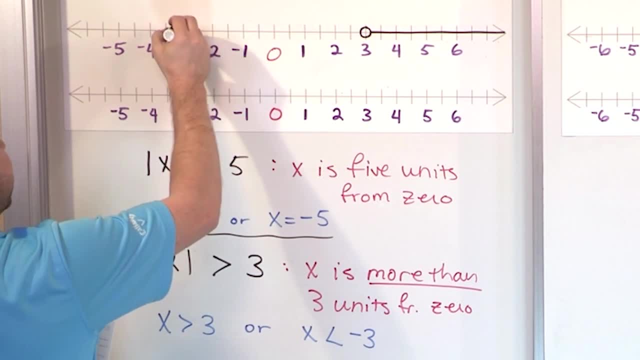 But X less than negative 3 would be an open circle at negative 3 and all the values to the left. like this, All the values to the left, Alright. So because of that, remember what the original absolute value is saying is, whatever X is. 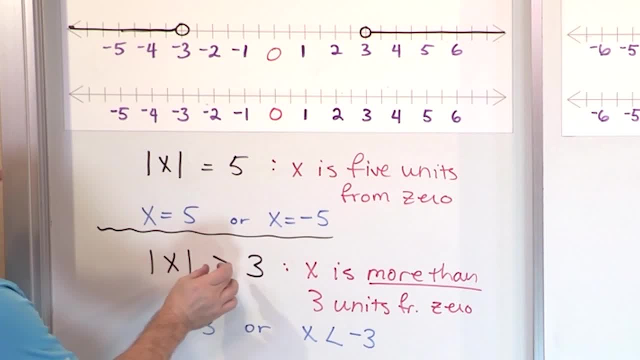 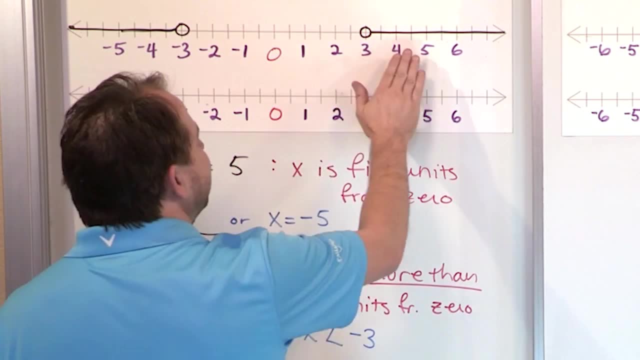 it has to be, because its absolute value is here. it has to be more than three distance units away from 0.. That's what it's basically saying. So we translate that to this graph: This is, of course, more than three distance units from 0.. This is more than. 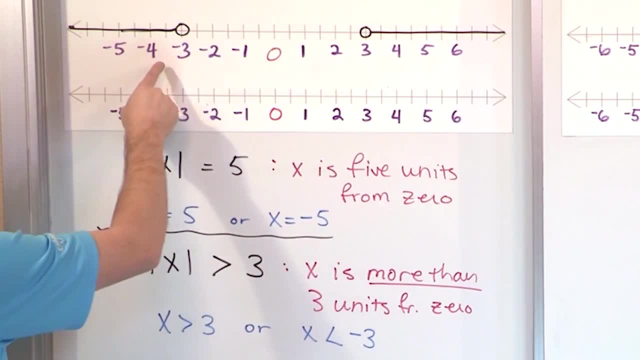 three distance units from 0, and so on, and so on, and so on. But when you look at the negative side, this negative 4 is more than three distance units from 0, and the negative 5 is more than, and the negative 6 is more than, and so on. 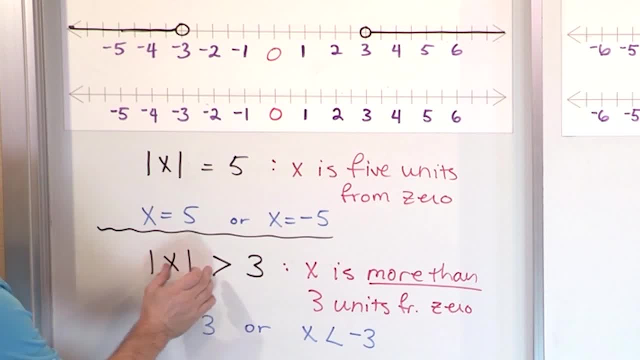 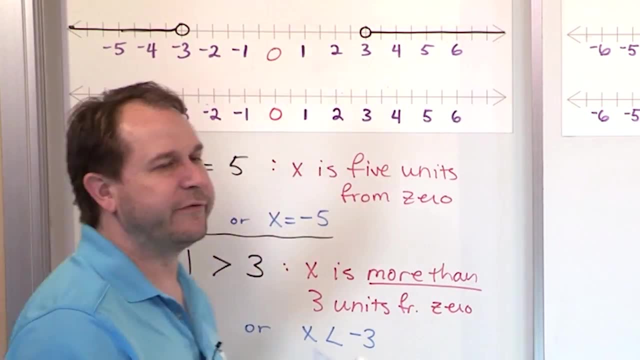 So when you see an absolute value of something bigger than a number, you need to mentally think of this. on the number line It's going to be bigger than three units away from 0. So when you see a greater than sign with an absolute value, 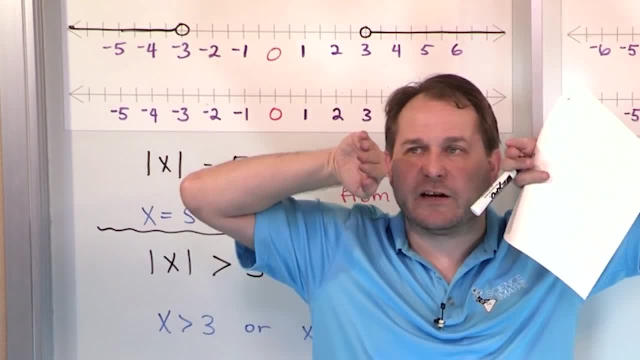 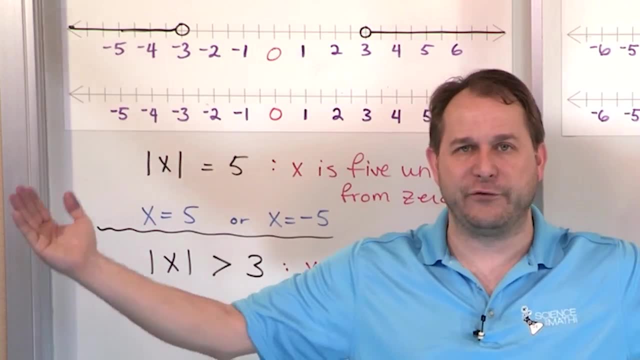 bigger than some number, then it means on the number line it's going to be, it's going to be a shaded region on the number line, larger, extending on to positive and negative infinity, away from two points, Because all of the points here that make up X have to be three distance units or more than three. 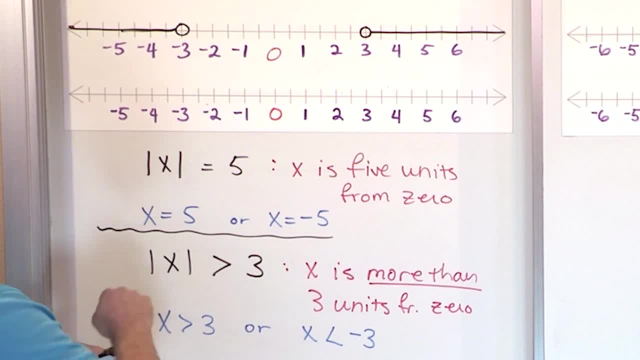 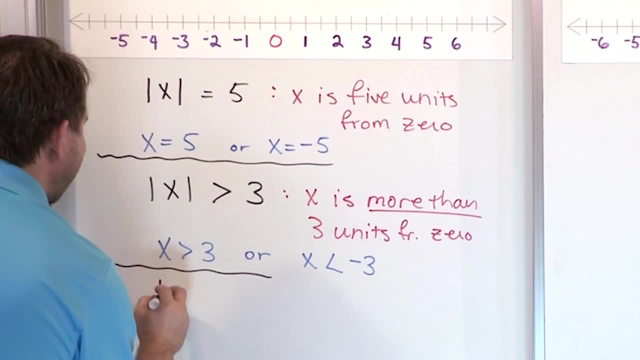 bigger from away from 0.. Now let's put the third case on the line, and then we'll be able to compare them and make it much, much simpler. The third case would be if you had the absolute value of X less than a number, And let's pick a different number to make it easy. 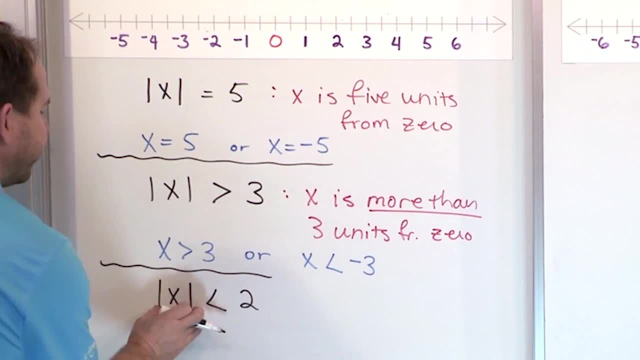 Less than two. What does this mean in English? It means remember. absolute value means distance from 0.. It means the set of points X have to have a distance from 0, that's less than two units away. So let's write that down before you go any farther. 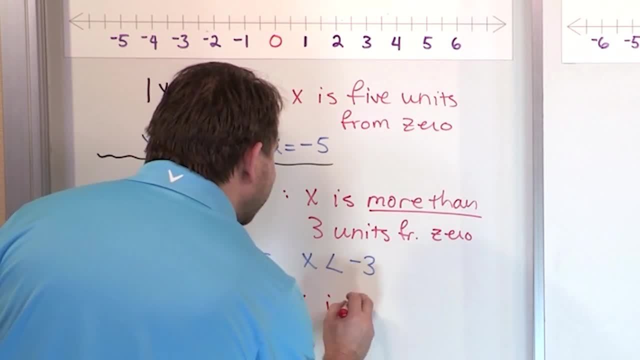 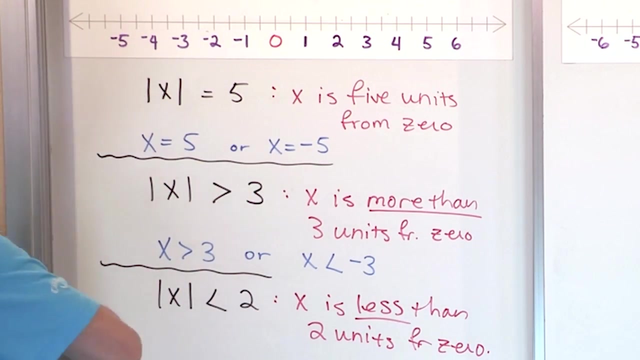 What that means is X. the set of points X is less than less than two units from from what? From always, from 0, right. So what that means in terms of you know writing it out like we did here it. 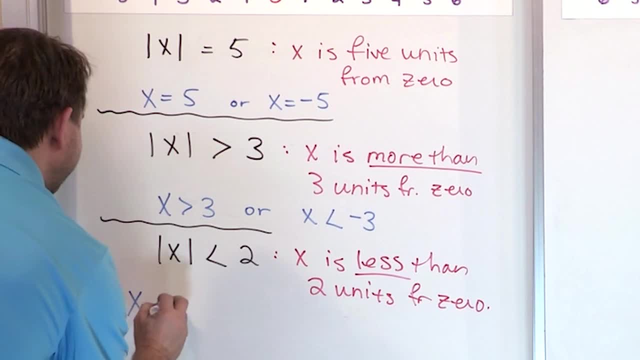 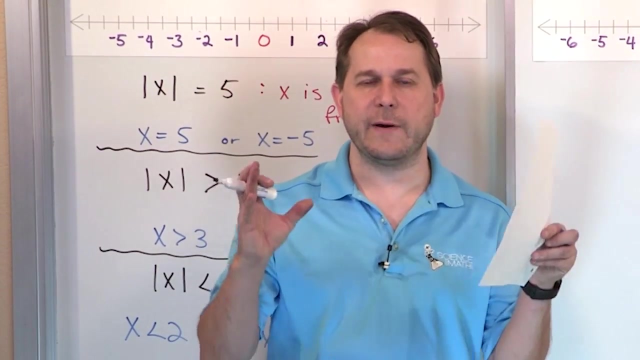 basically means that X can be less than two, but X also has to be greater than negative two. That's, I'm doing a translation. It's like it's like going from Russian to English or French to Spanish or something. You have the absolute value. 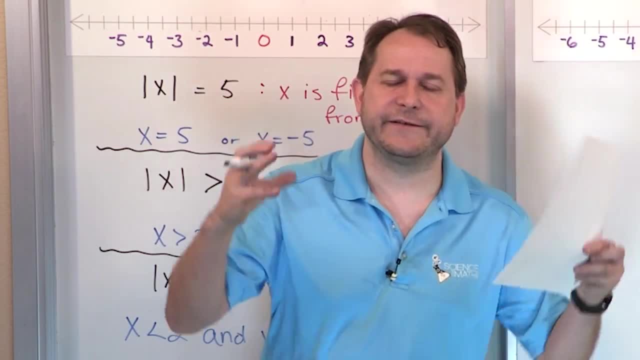 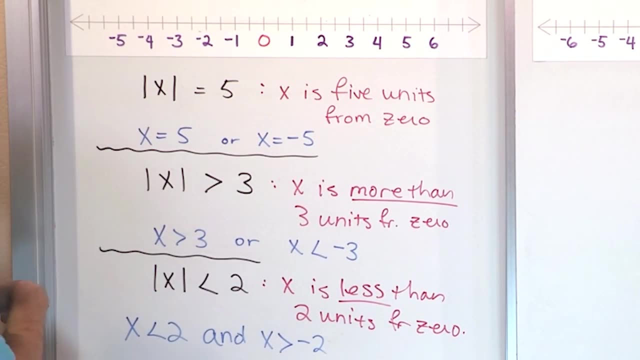 problem, but you have to in your mind understand what it's saying so that you translate it into these two separate equations, because you already know how to solve these equations and how to plot them. We've been doing that before. So the only step here with the absolute value inequalities is taking this and 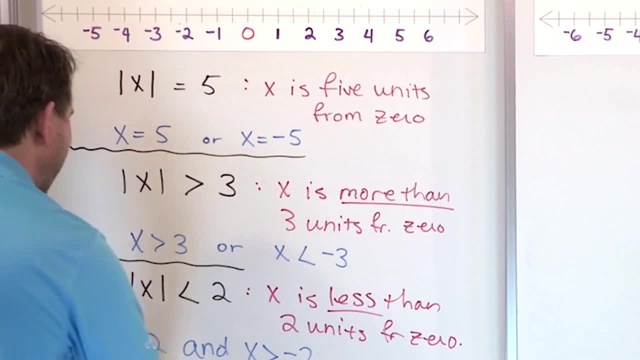 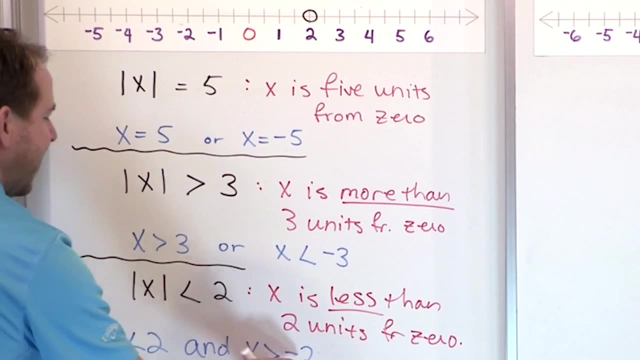 translating it into English. So let's see why this is the case. X is less than two. It means I put an open circle here at two and it's going to be the numbers less than But and X is greater than negative. two means I have to put an open. 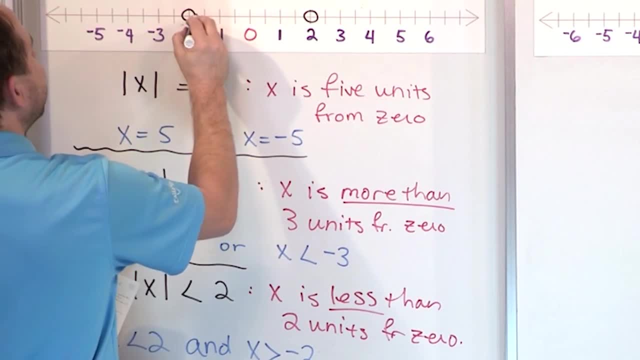 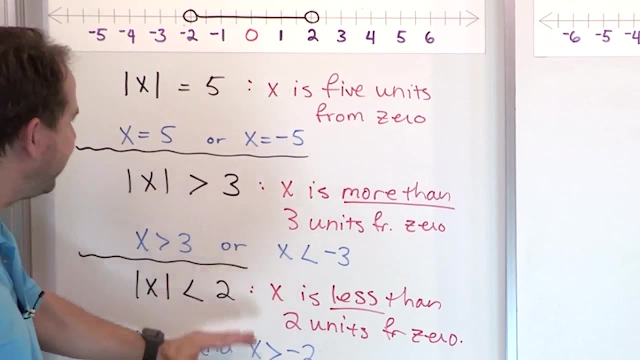 circle here, So it has to be greater than negative two and less than two. So it's this line segment, right? So now you see what it means. It's when you have an and it's a segment on the number line, just like before When you have an, or it's. 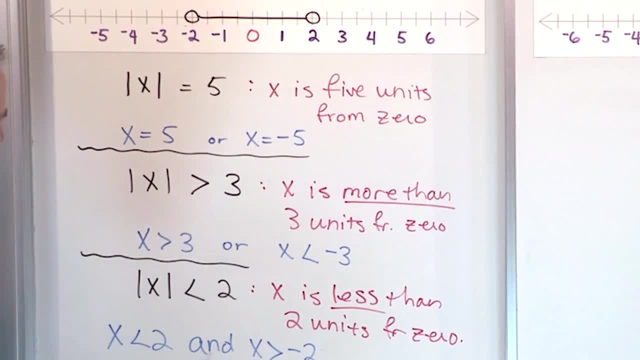 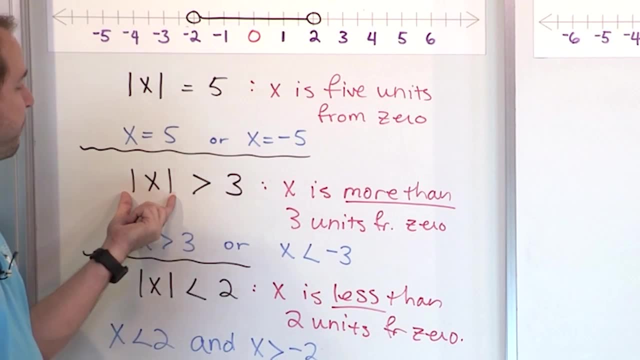 going both directions from some points, just like before. The only new part of the, the, the wrinkle, is that you need to start to remember that when you see an absolute value of X or some expression of X greater than a number, it's basically an or type of problem. And whenever you see an absolute value of X, 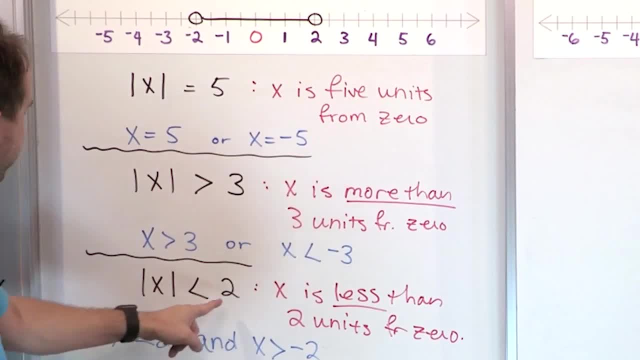 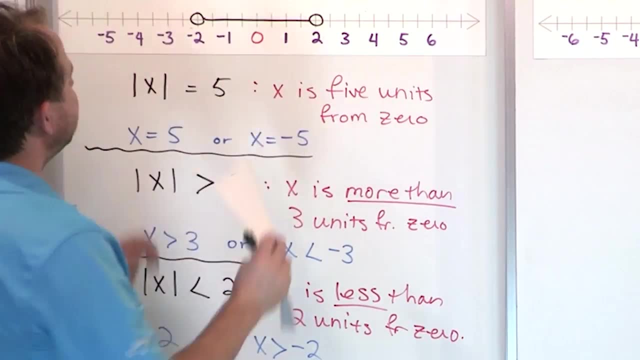 less than a number. you need to think of it as distance from zero has to be less than two units, So it has to be a region symmetric. you know, with zero in the center, That's two units to the left, two units to the right, because that's what. 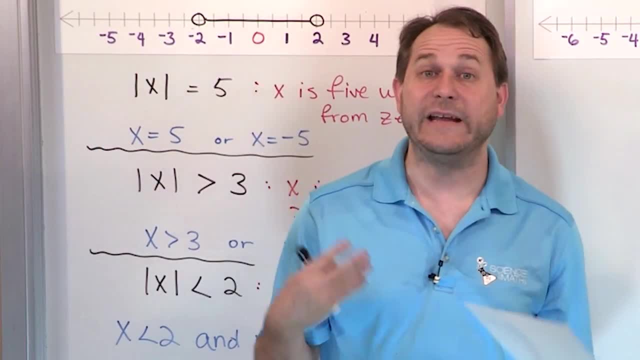 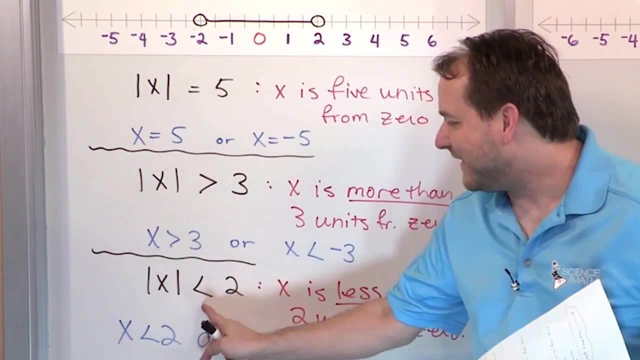 that means. So it's a little hard in the beginning to read those problems and say, oh, yeah, yeah, that's going to be this. But as time goes on you will start to realize when you see an absolute value less than some number, it's going to be a segment. 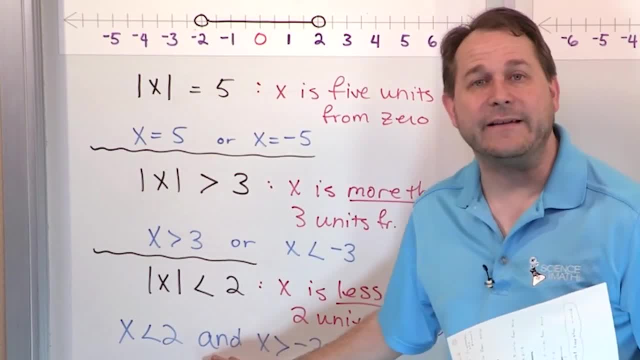 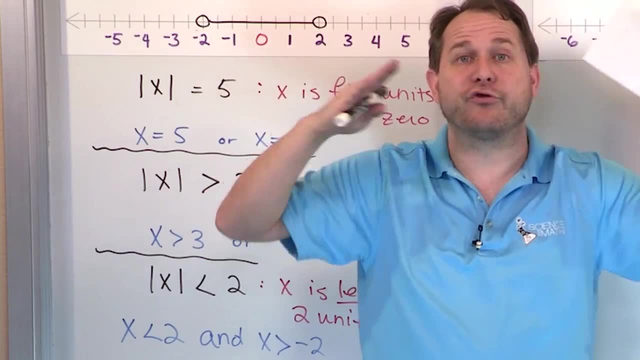 on the number line and means it's going to be an and kind of deal, And whenever you see absolute value greater than a number, it's going to be extending on to positive and negative infinity, both directions, as the or problems have been doing in the. 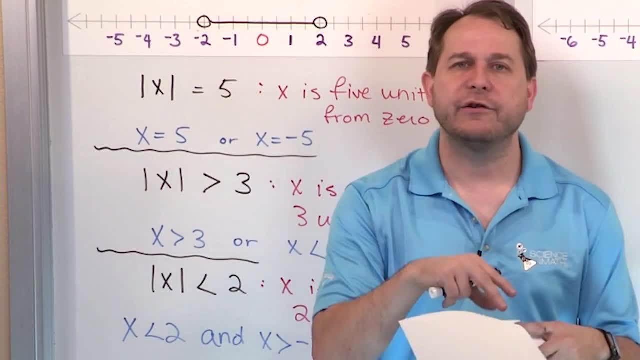 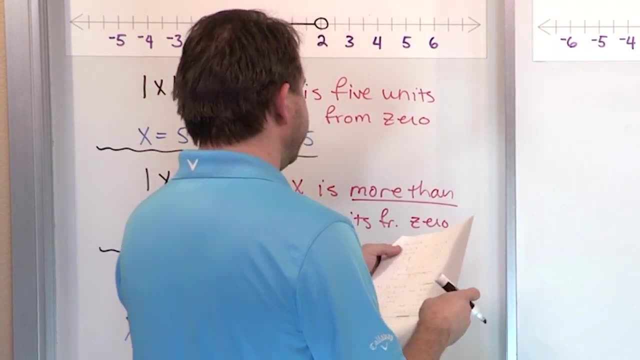 past. So I think the best way to proceed is: I want you to try to remember these cases. But the best way to proceed is let's go ahead and do a few problems and graph them and you'll get some experience as we go on. So probably the easiest one. 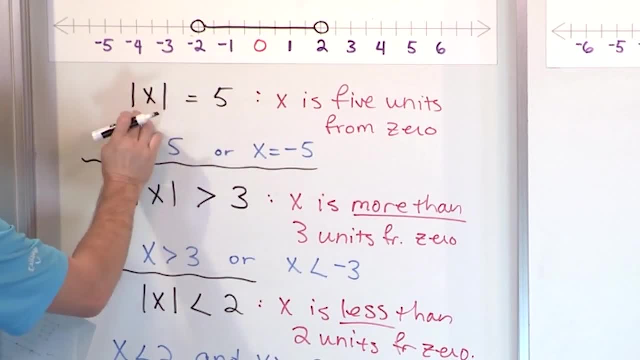 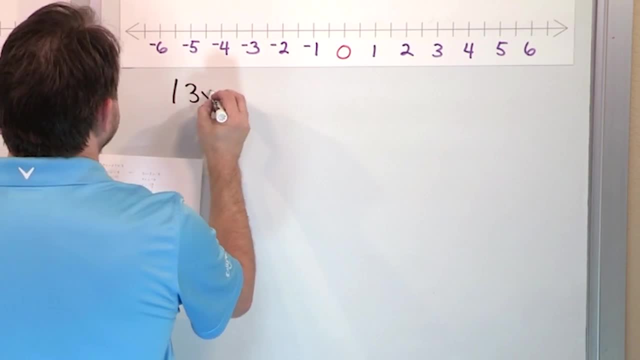 we can do will look similar to this one right where we had an absolute value of something equal to a number. So let's do one like that really quickly and see what we get. Absolute value of 3x minus 2 equals 8.. Now what this means is that, whatever 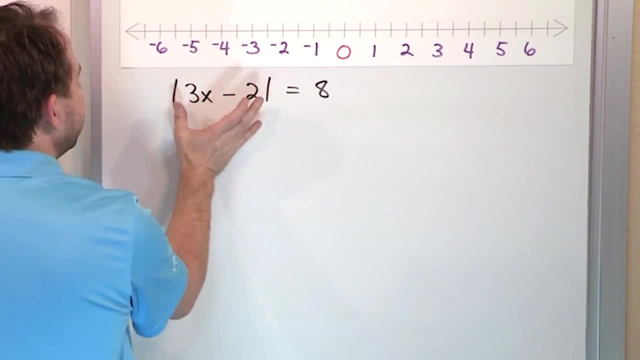 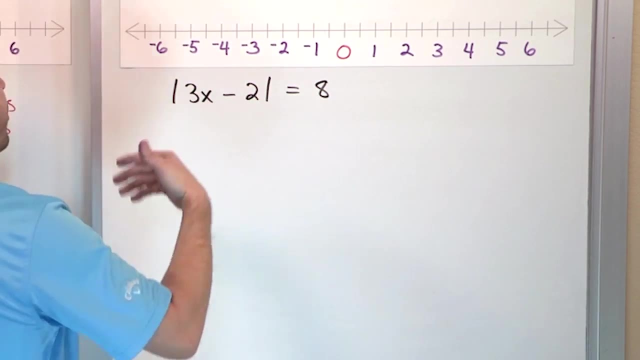 goes in this absolute value here. whatever this expression is, I have no idea what it is because it has a variable, but whatever it is, whatever is inside of here, can either be a positive 8 or it can be a negative 8, because once I take its absolute 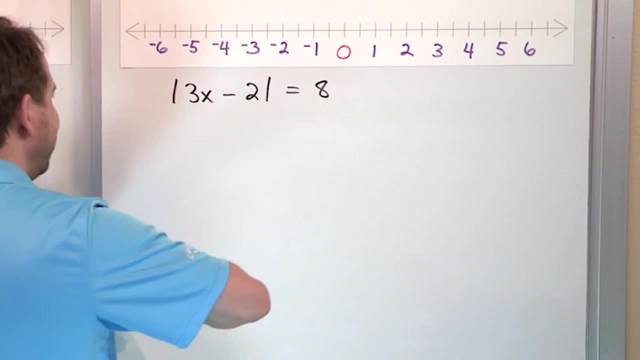 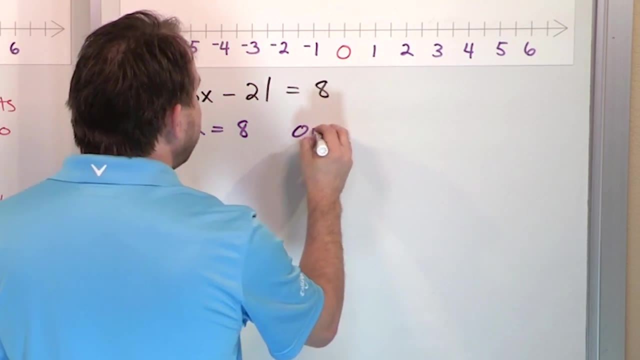 value, it's going to give me 8.. So you always are going to kind of get two little equations out of this. What you're saying is: 3x minus 2 can definitely be equal to 8.. Of course it can, Or it can also be equal to negative 8.. Why? Because if I replace 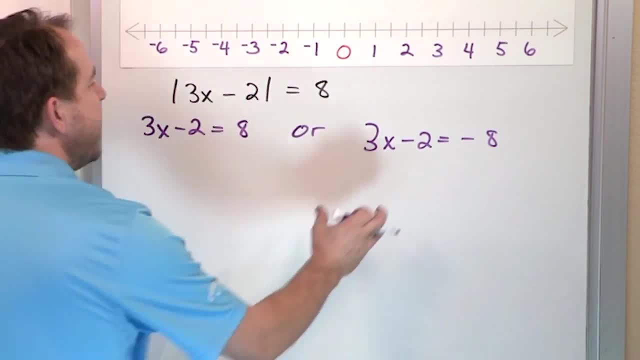 this with 8 and take its absolute value, I'll get 8.. If I take and replace this guy with a negative 8, I will take its absolute value and I'll still get 8.. So I can make it equal to positive or negative 8 and then I just solve them separately, So moving. 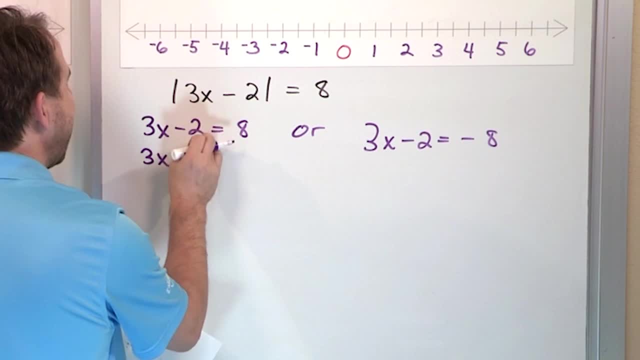 the 2 to the other side, 3x equals. when I add 2 to both sides, I get 10.. And when I get x by itself, it'll be 10 thirds, just dividing both sides by 3.. So this, or let's. 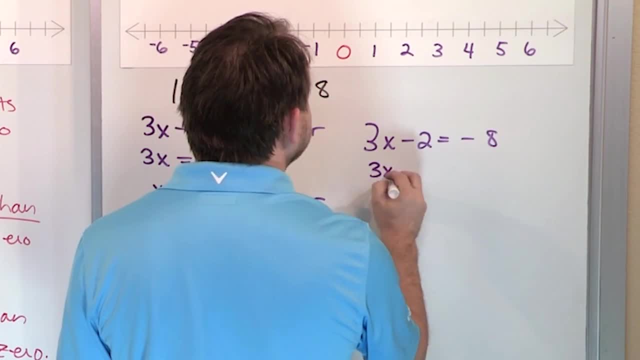 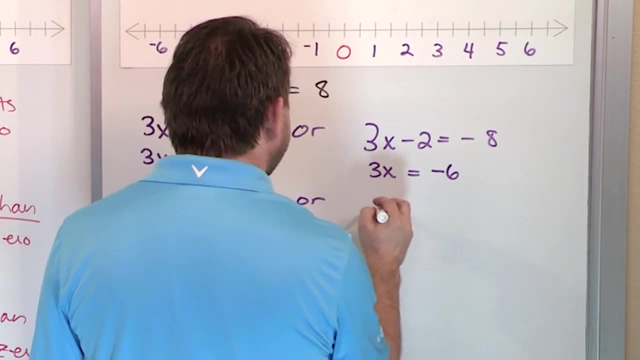 solve this side. Adding 2 over here, I'll get 3x equals what is negative? 8 plus 2? You'll get negative 6 on the right-hand side. If I divide by 3, I will get negative 6 thirds. So that means that x is going to be equal to negative 2.. So that's the. 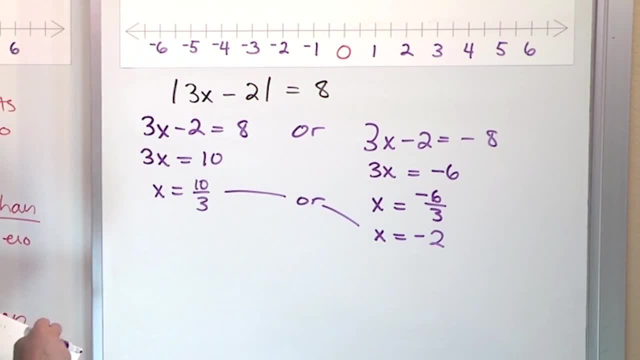 answer. So what I figured out is that there's an or here between these guys, because this inside of this can be either plus 8 or minus 8, so the or kind of ripples down to the bottom. So what we're basically saying is that this, this absolute value equation. 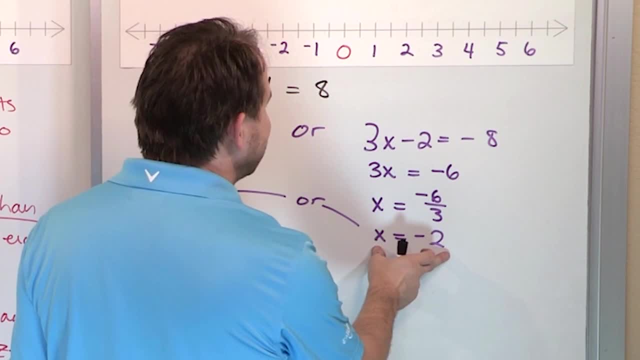 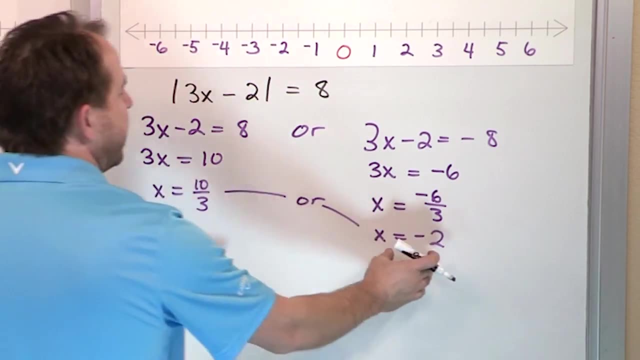 has two different answers. One of the answers is if we put a negative 2 in there, and the other answer is 10 thirds. So if we plot them on the number line, what we're going to get is we're going to have a dot at negative 2, and then we'll have another dot at 10. 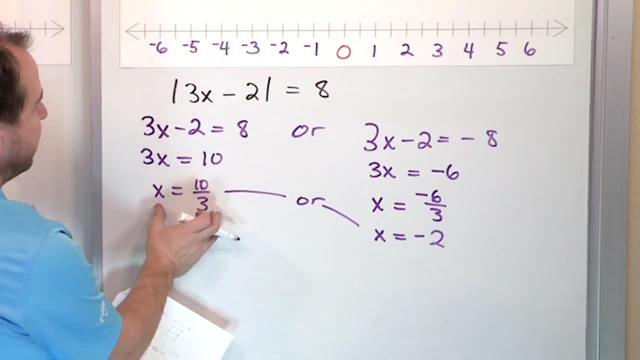 thirds. So that's basically 3.33.. If you divide that out, it's 3.33,, which would be here's 3, here's 4, so it's basically going to be somewhere around around here And there's. 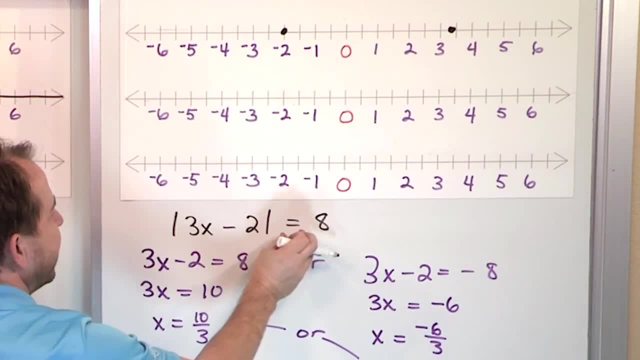 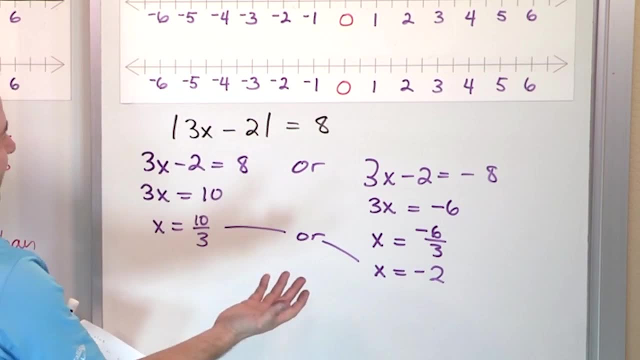 two points, only two points. There's no range of values because there's an equal sign here instead of an inequality, And you can always check yourself. Put negative 2 in here. What do you get? 3 times negative 2, negative 6, minus 2, negative 8.. Take its absolute value. 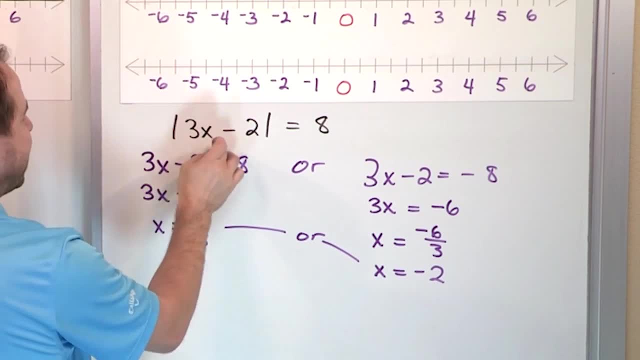 you get an 8. Stick a 10 in here 3 times 10 thirds. the 3's will cancel. you'll get 10, minus 2 will give you 8.. Take its absolute value, that will give you 10.. So that's. 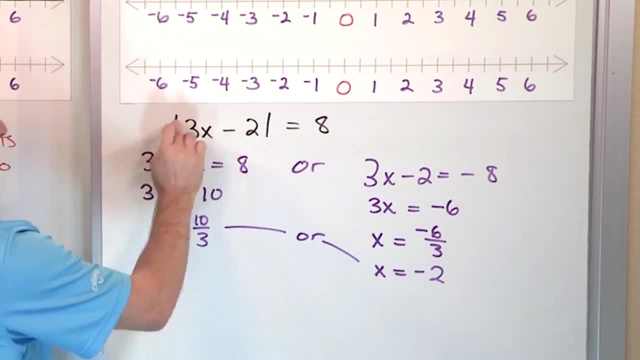 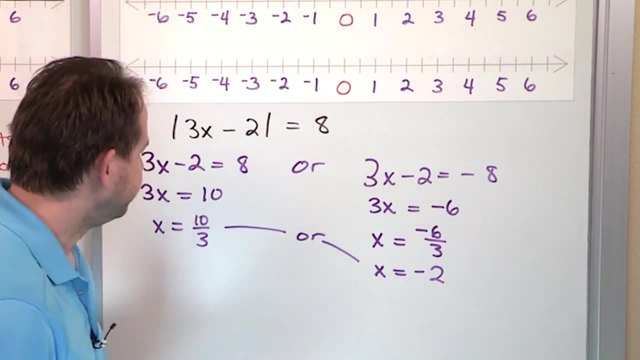 the absolute value that will give you the 8.. That's why you have two answers, because the whole entire thing on the inside can either equal 8, or it can equal negative 8.. Both are going to give you the same exact answer. 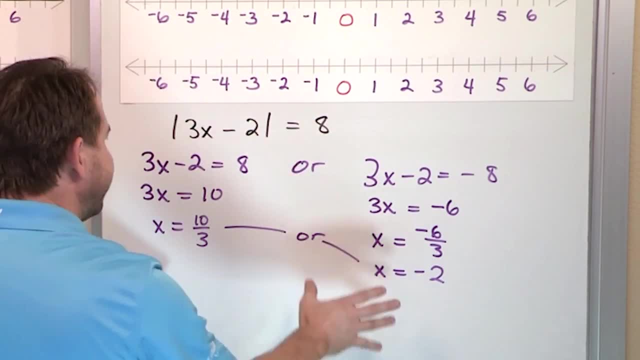 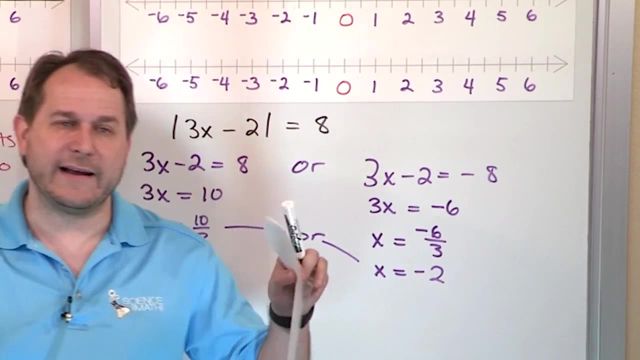 Alright. So typically when we do these things, we kind of introduce by showing some simpler problems like this one, But typically what you'll have is inequalities greater than something or less than something, and then you'll have to translate it, as I said, using one of these. 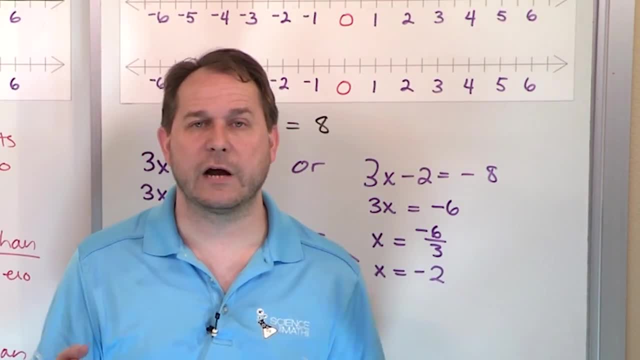 rules into an AND or an OR, kind of compound inequality, and then something like that. So you'll have a compound inequality and then solve it the same way as before. So as we solve the next problem, keep in mind, if you see, the absolute value of something. 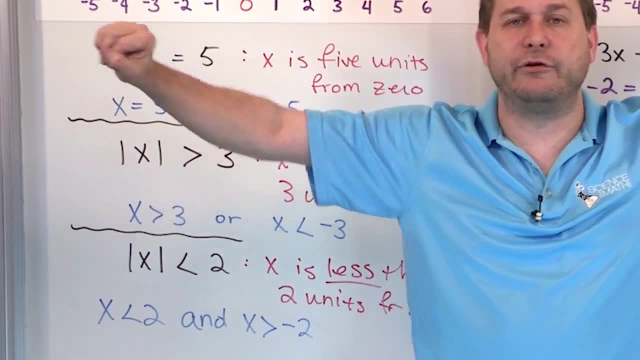 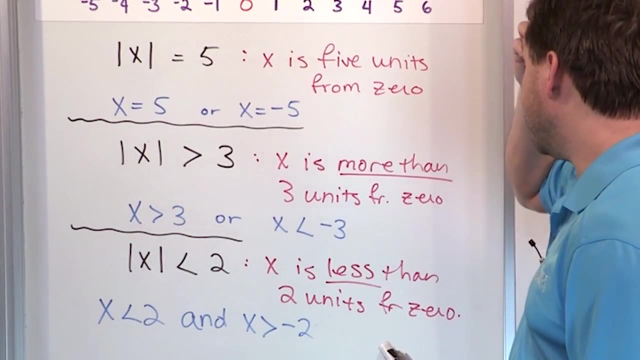 bigger than a number, it means it has to be that many distance units or more away from 0. So you're going to have, you know, shaded regions going away from the origin. And if you have an absolute value of something less than a number, it means you're going to have 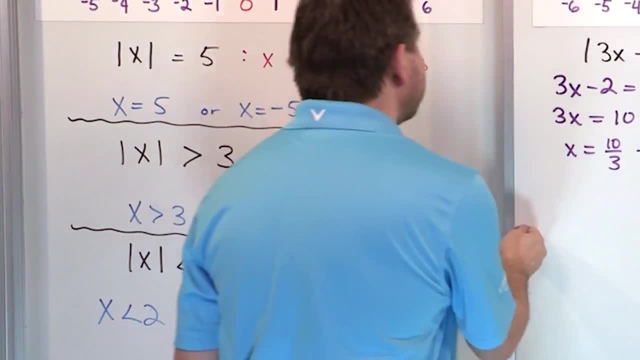 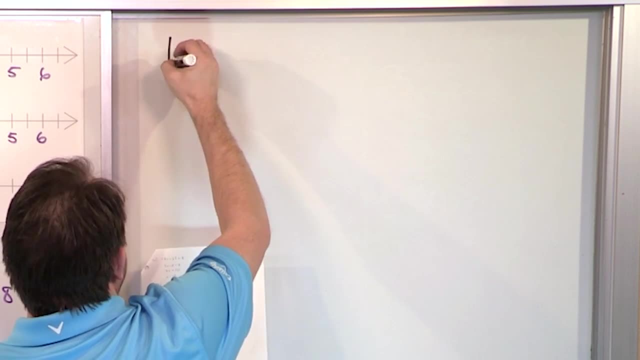 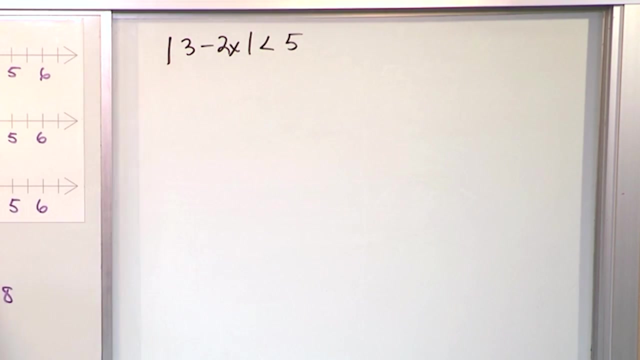 a shaded segment that's centered around the origin. So let's go ahead and see that in the next problem. So what we're going to have for the next problem is going to be absolute value of 3 minus 2x less than 5.. So immediately you need to try to categorize. 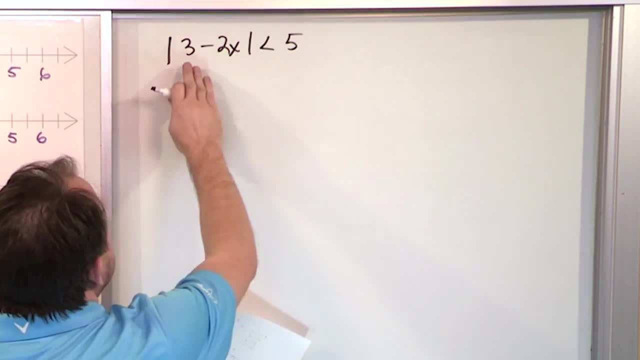 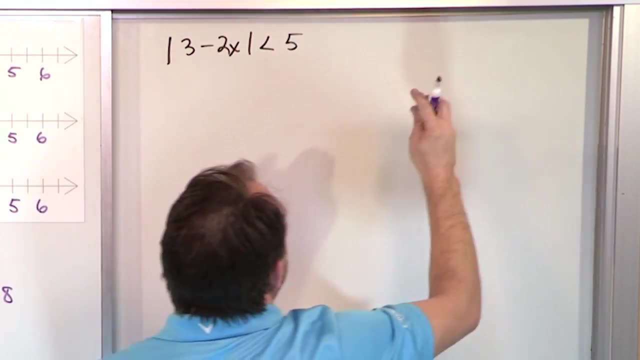 this and try to figure out what it's going to look like. Now, I know that this doesn't say x, It says 3 minus 2x, But still it's some expression of x inside of this and it's less than a number. So if you can think in your mind what we just said, to remind ourselves, 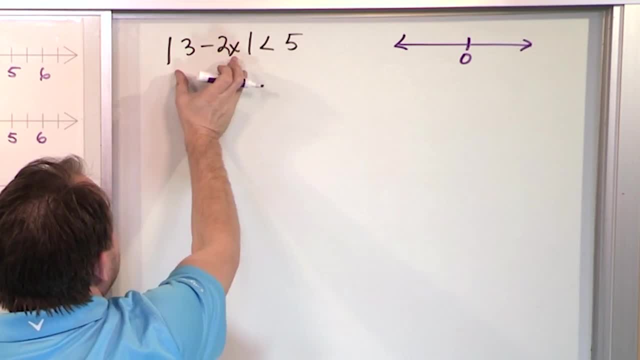 is. this is 0.. If this were x, it would be: whatever this is has to be less than 5 distance units from the origin. So if that's 5, it's less than a number. And if this were x, it. 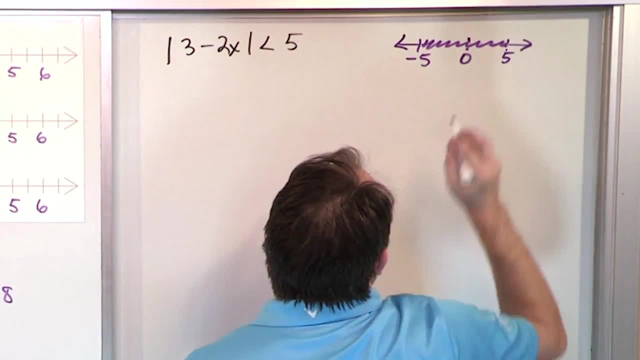 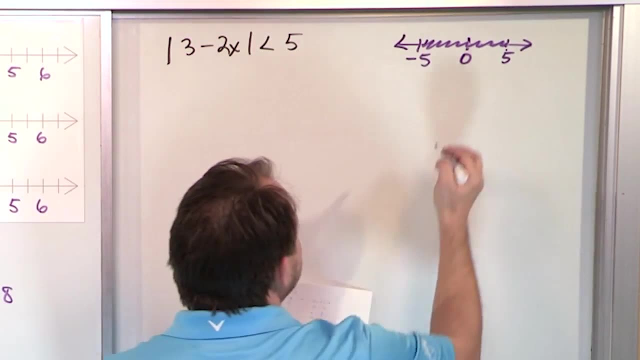 would be less than a number And that's negative 5.. Then 5 distance units, plus or minus 5 distance units from the origin means it's going to be a line segment shaded there, which means it's going to be an AND kind of deal If this were flipped the other direction. 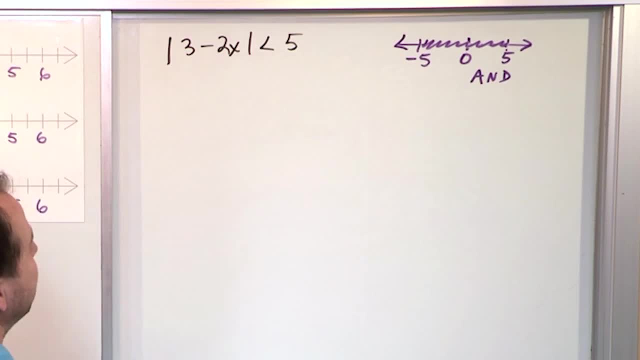 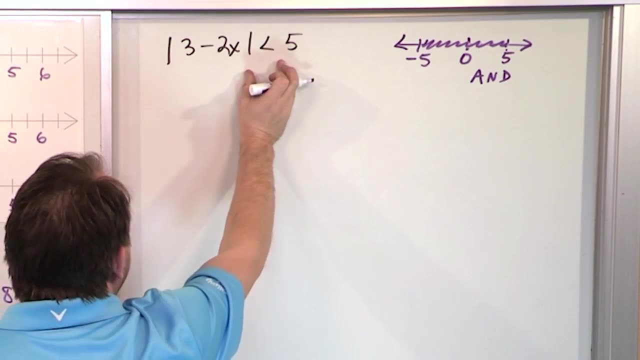 greater than then, it would be an OR and it would be shaded both directions out to plus or minus infinity. But what you're saying is what's in here has to be 5 distance units away or smaller from the origin. So that's exactly what we have shaded here. So let's 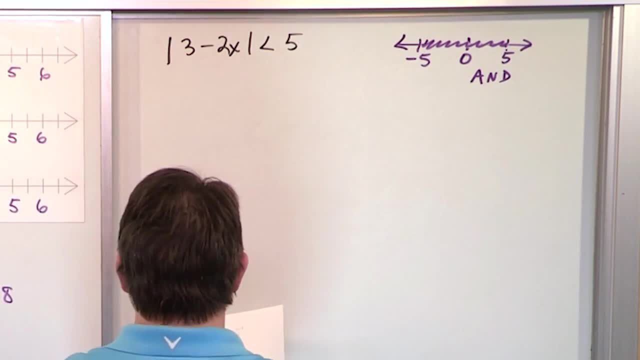 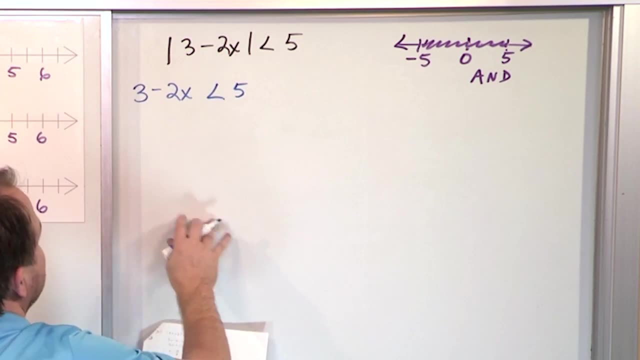 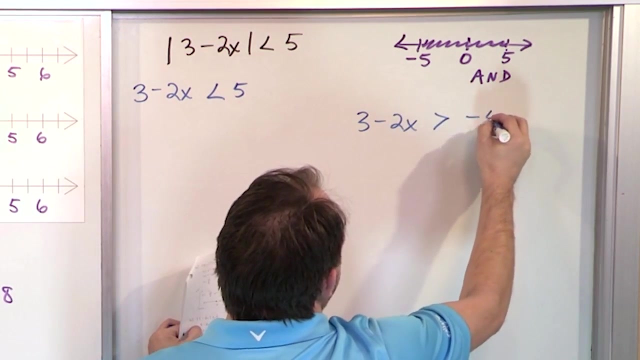 go ahead and solve the rest of it. Now that you kind of put it into words, now you can rewrite it and say we have two inequalities: 3 minus 2x, It is going to be less than 5, but also- I guess I'll go down over here- 3 minus 2x can be greater than negative 5.. 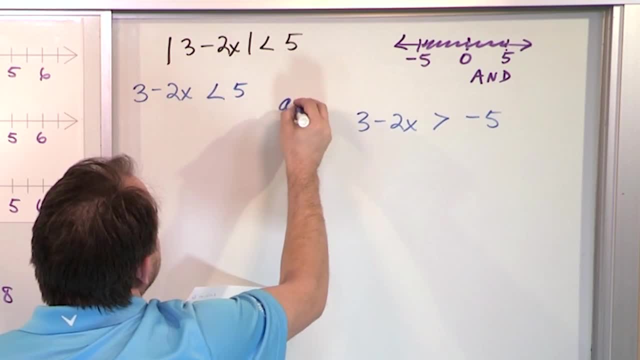 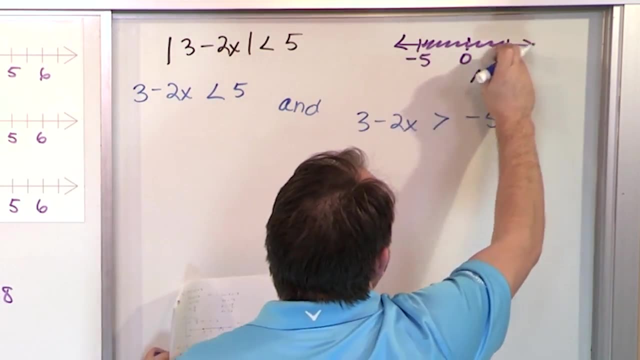 Look at what I've written here. It can be less than 5, but if I join them with an AND, it can be less than 5 but greater than negative 5.. So this quantity can be greater than negative 5 and less than 5, at the same time forming a segment there. I've translated this to English. 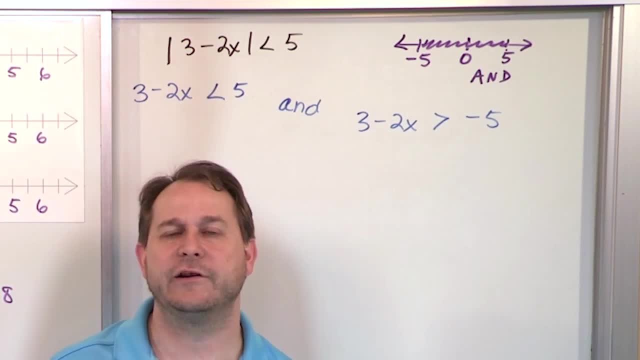 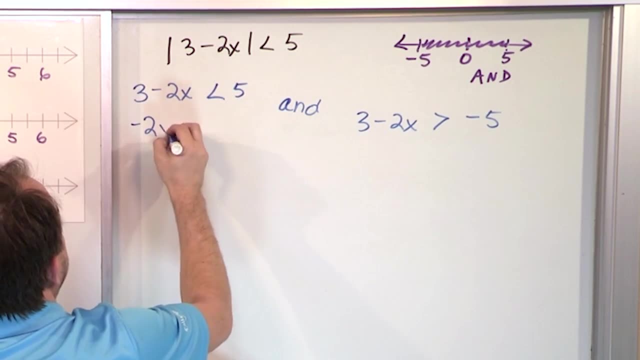 and now the problem becomes exactly what we've done in the last section: just solving those again and again, because we've done a lot of them. So let's move the 3 to the other side. We'll get negative 2x less than subtract 3, subtract 3, we'll get 2.. And then x. now 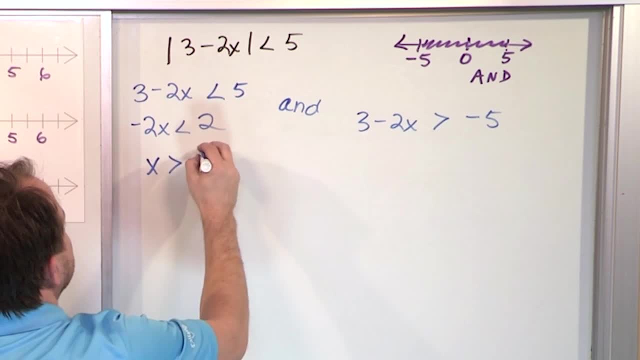 we're dividing by negative 2, so we'll have to flip the direction of this 2 over negative 2, so x will be greater than negative 1.. That's going to be one half of the answer. The other half of the answer will be over. 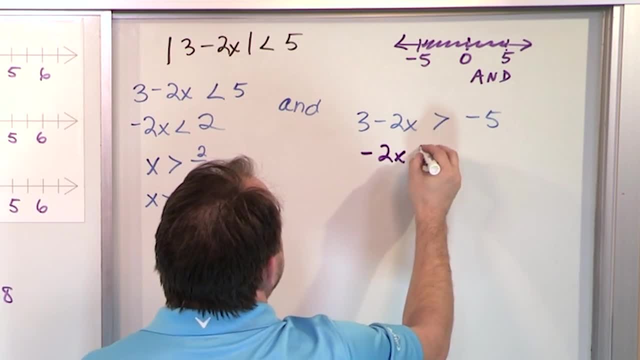 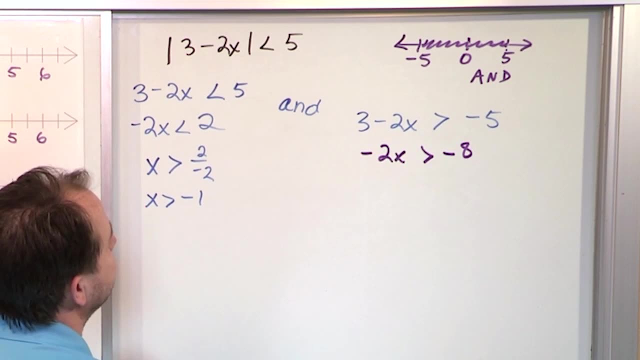 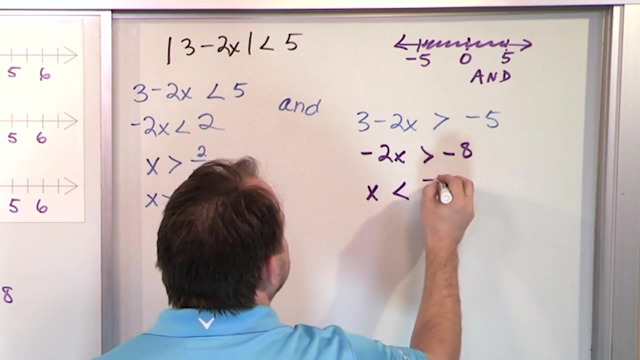 here. Move the 3 over here by subtraction. Negative 2x greater than what is negative 5 minus 3? Negative 5 minus 3 will be negative 8.. Right Now we get x by himself, but we divide by negative 2, so we have to flip the direction of our arrow. Negative 8 divided. 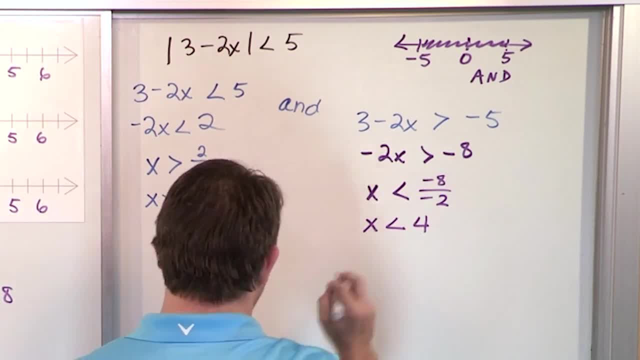 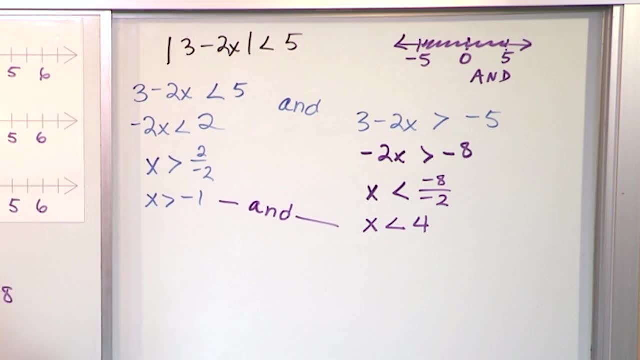 by negative 2,, so x will be less than positive 4.. And since there's an AND here, this is joined by an AND as well. Both of them have to be true in order to form a line segment like that. And since they both have to be true, we can stick and rewrite it again in: 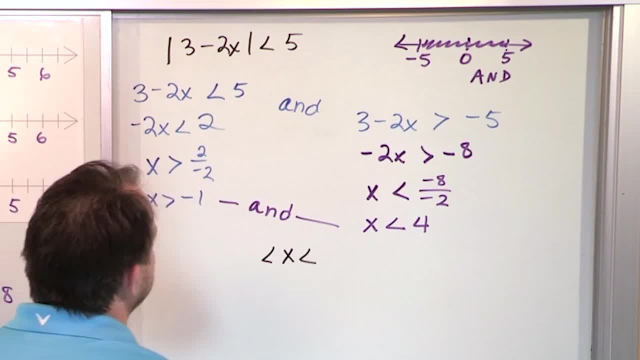 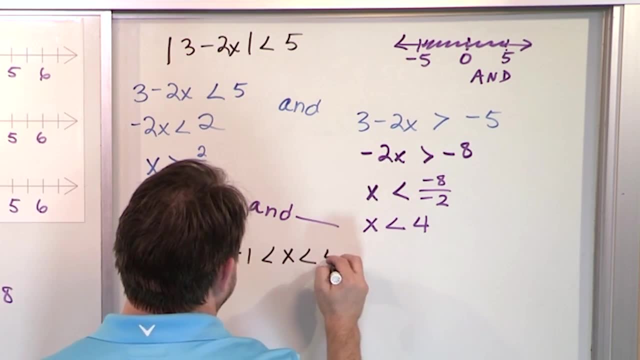 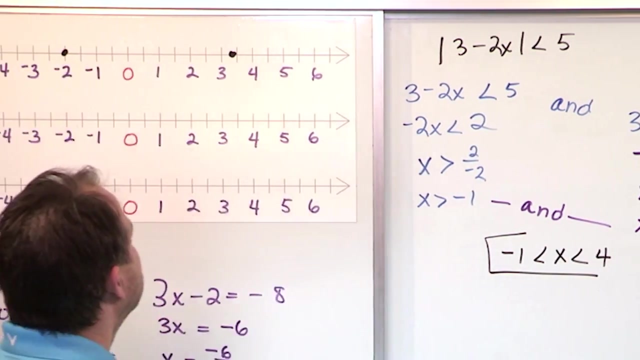 our other notation, x, we'll put our less than signs in both places: x is greater than negative 1.. x is less than 4.. So this is what you would circle on your test: x is greater than negative 1 and at the same time less than 4.. But if we come over here we can say: 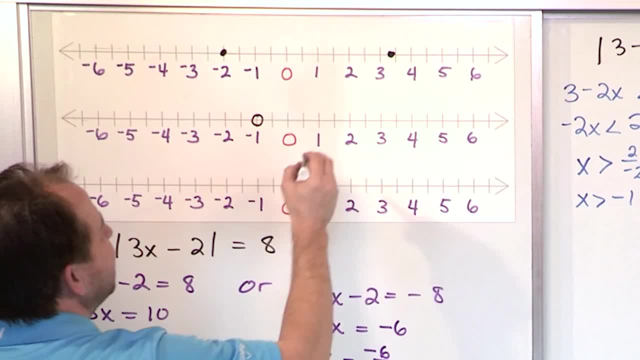 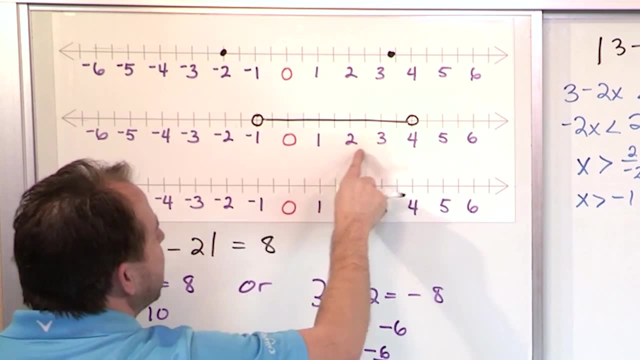 less than negative 1, or I should say greater than negative 1, at the same time, less than 4 means it's a segment that extends between these two, between negative 1.. So it's greater than negative 1, at the same time being less than 4.. Greater than negative 1, less than 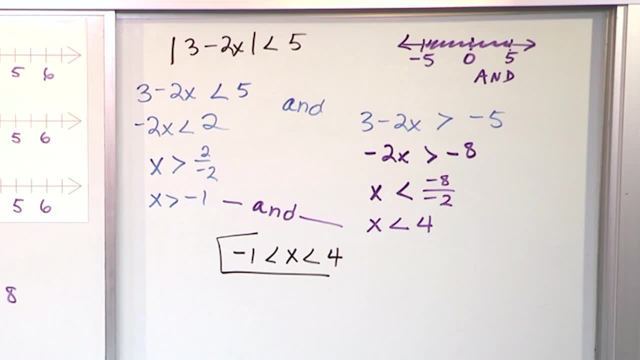 4. So it forms this line segment with two open ends at the end. So literally everything in this section boils down to you being able to translate the problem from what we had before into two inequalities which we already know how to solve. from the last section. 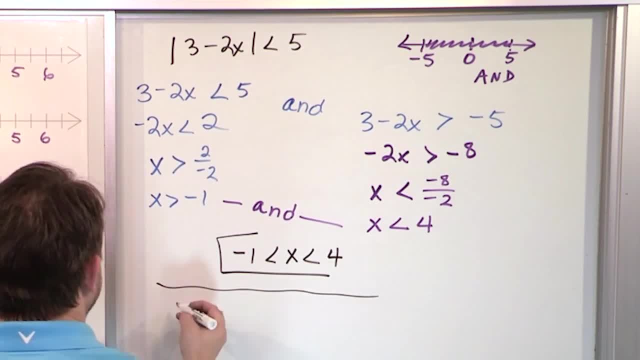 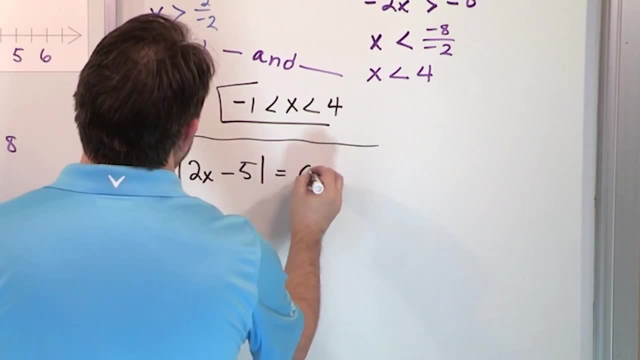 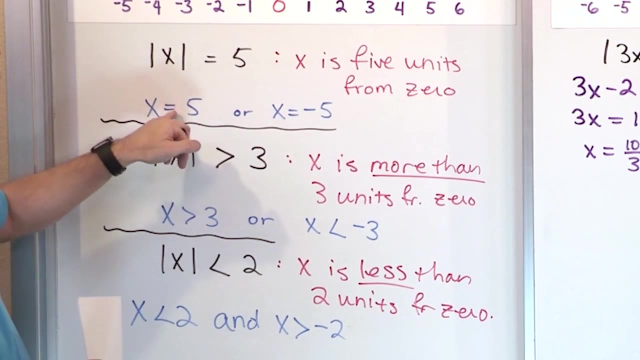 All right, let's do this next one. This one's pretty good, I think. to illustrate a point: 2x minus 5, absolute value equals 0.. Now we had a similar set of problems. We said when we had an absolute value equal to a number, it would be it could say the inside is equal. 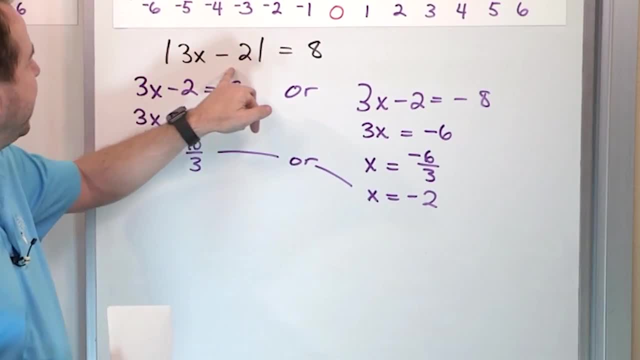 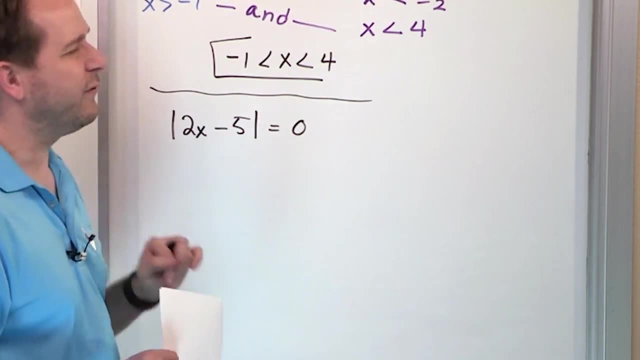 to 5 or negative 5.. We actually did one here. We said the inside could be equal to 8 or the inside could be equal to negative 8.. But this is why I wanted to do this problem. Now we have an absolute value equal to 0. Well, there really is no such thing as an absolute. 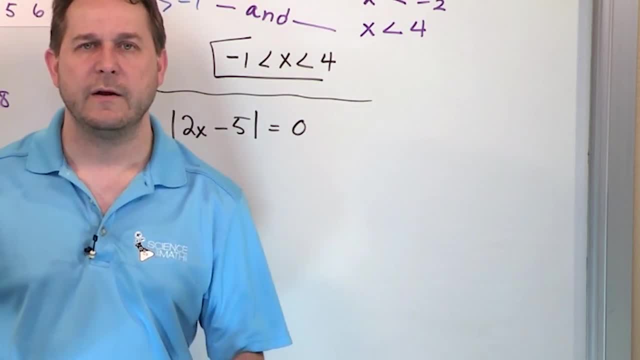 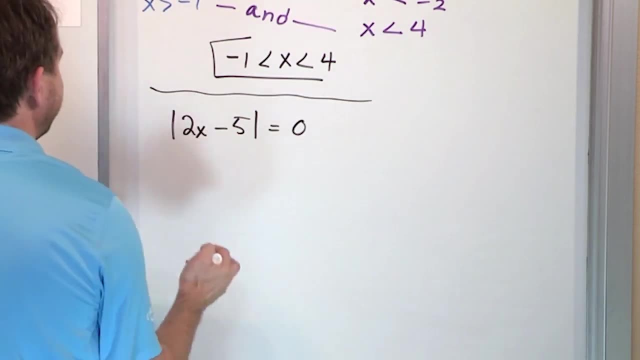 value equal to 0. There's no such thing as negative 0 and positive 0. 0 is right in the middle. So really there's only one equation here. When you have an absolute value equal to 0, there's really there's not two different things to pull out of it. Basically, there's. 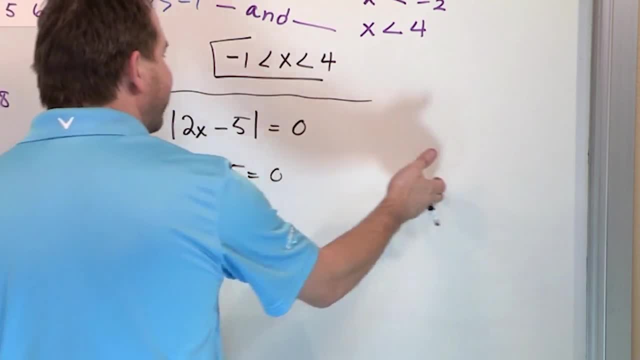 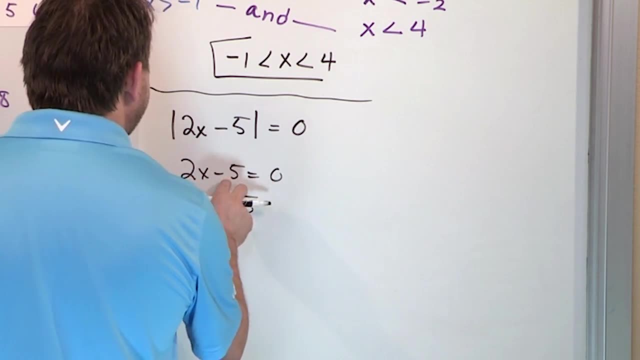 only one. 2x minus 5 can be equal to 0. You can't have a negative 0 and a positive 0. There's just one 0. So there's only one equation: Move the 5 over making 2x equals 5, just. 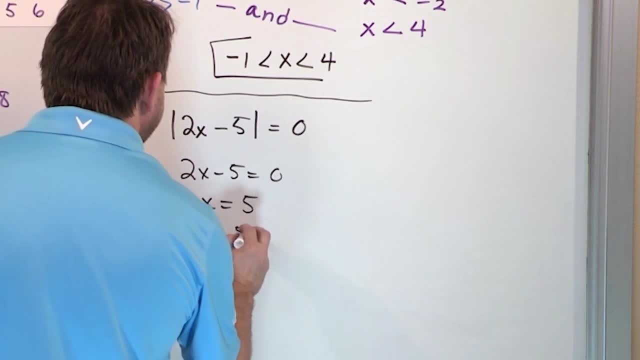 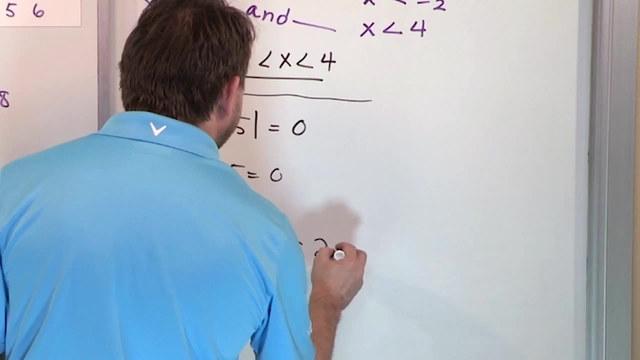 by adding 5, adding 5.. And then x is going to equal to 5 halves, because we divide by 2, divide by 2.. So what we basically said is 5 halves, which, as you know, is 2 and a half, or I guess is. 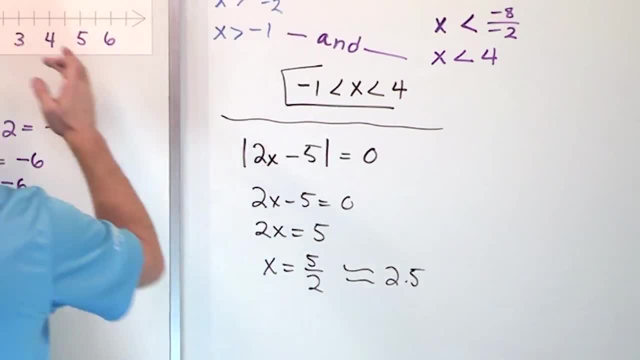 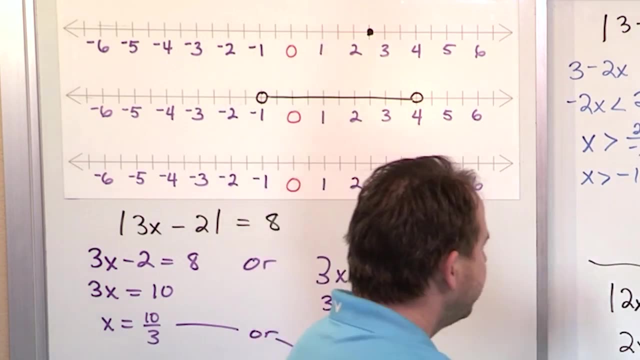 exactly equal to 2 and a half. So if you were to go in the number line here, let's just erase this one, since we don't need this anymore. 2 and a half is basically right there and there's only one value that works. So if you put 5 halves in here, 2 times 5 halves the 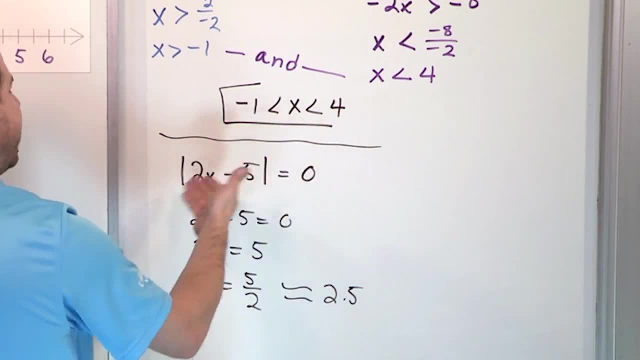 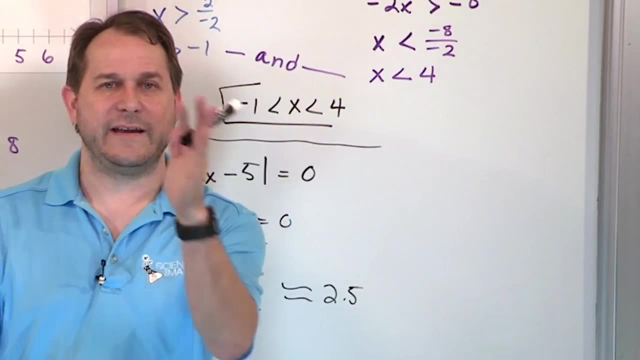 2s will cancel. You get 5 minus 5, which is 0.. Take its absolute value: you'll get 0. There's only one number that works. Absolute value usually gives you two answers, but when the number on the right-hand side of the equal is actually 0, then you only have one answer. 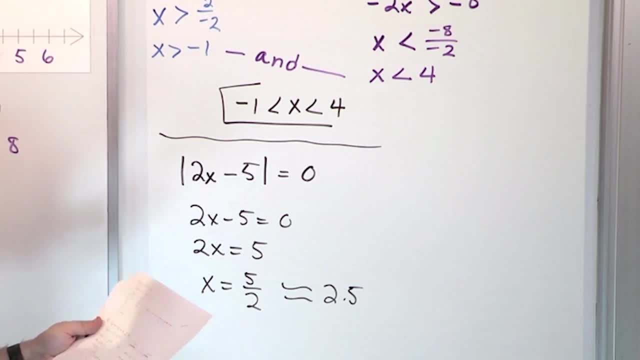 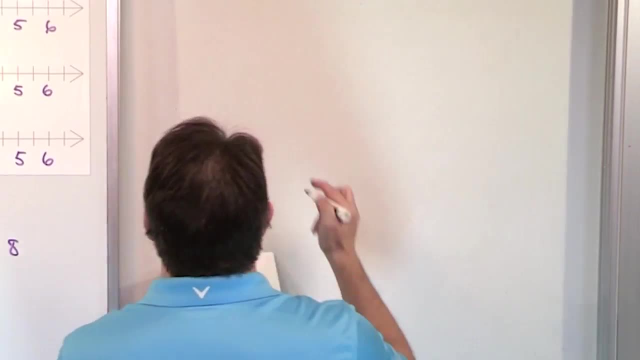 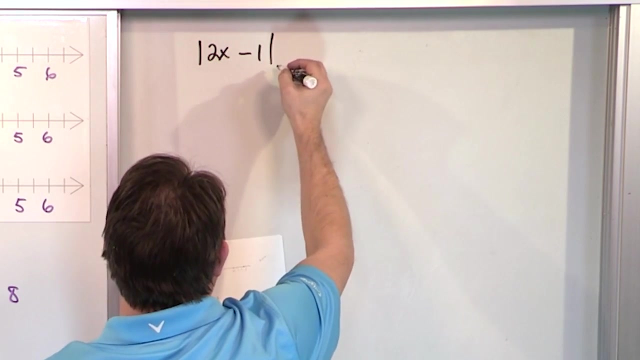 And that's why I wanted to do this one, to kind of show you that, All right, we have one more problem to do, Just to increase the complexity just a little bit. What if we had the absolute value of 2x minus 1,. absolute value closed plus 3? 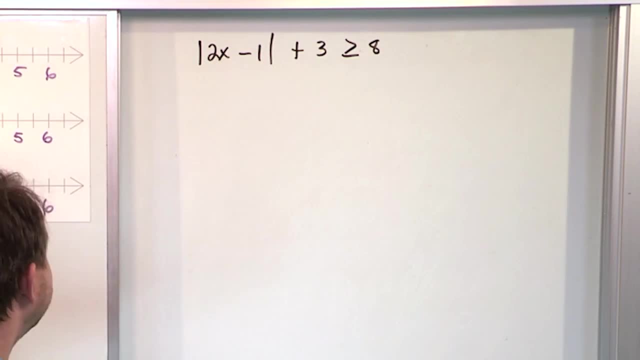 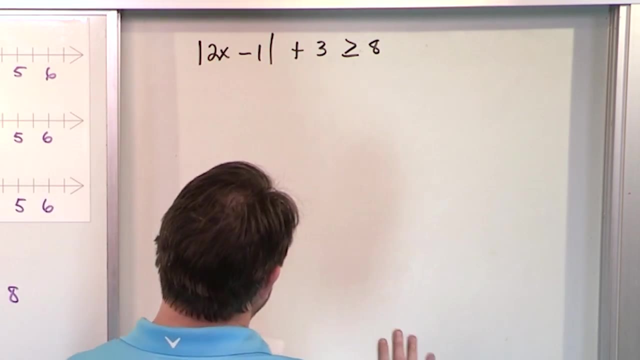 greater than or equal to 8?? Greater than or equal to 8.. So this is a little bit weird, because we have a number on the right-hand side of the equal, which is actually 0, and because we have a number outside of the absolute value. we haven't seen that before, But still. 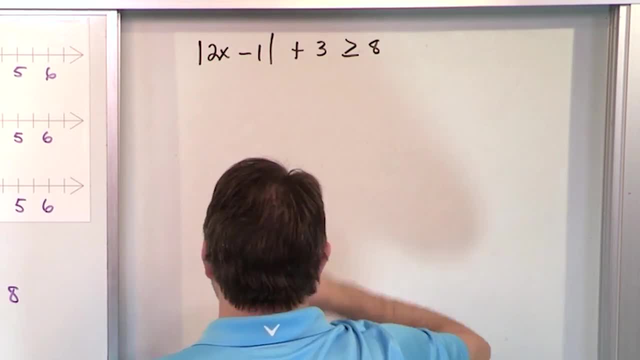 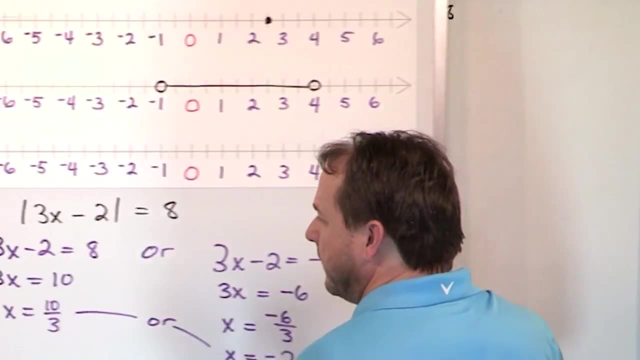 you have an absolute value on one side of the inequality and a greater than sign. So before you go any farther, I want you to, in your mind, try to think what it's going to look like, And we can go back to the beginning to refresh your memory, When we had an absolute 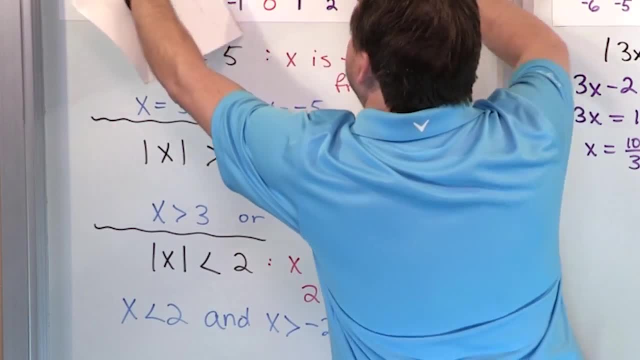 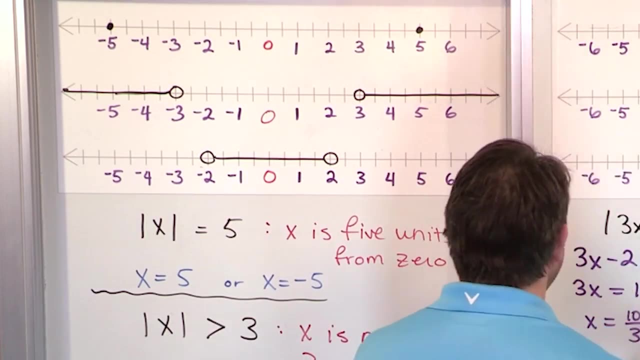 value greater than a number. then it ended up being an or, and it looked like this: When we had an absolute value less than a number. it ended up looking like a segment like this: which was an, and Now we have an absolute value greater than a number. 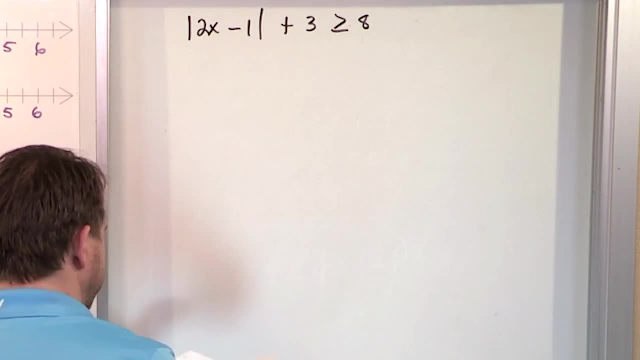 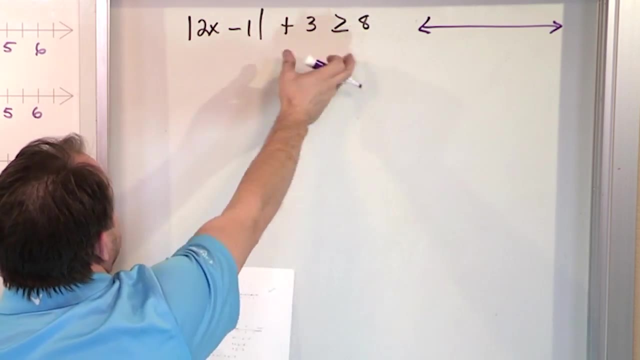 Now we have an absolute value greater than a number. Now we have an absolute value greater than a number, which means, if you were to kind of just think about it on the number line, whatever's on the left-hand side of the equal sign with the absolute, I'm sorry, the inequality inside of the inequality here is going to. 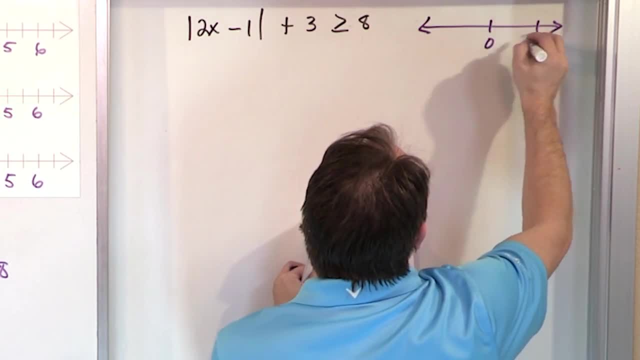 be greater than 8 units away. So if this is 0, and this is 8, and this is negative a, what we're saying is that whatever's in this inequality- yes, there's a 3 here, I know. 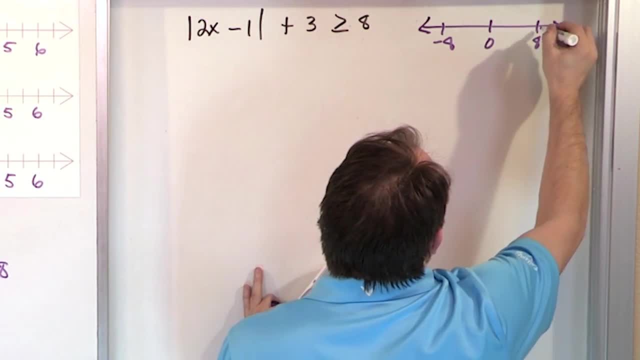 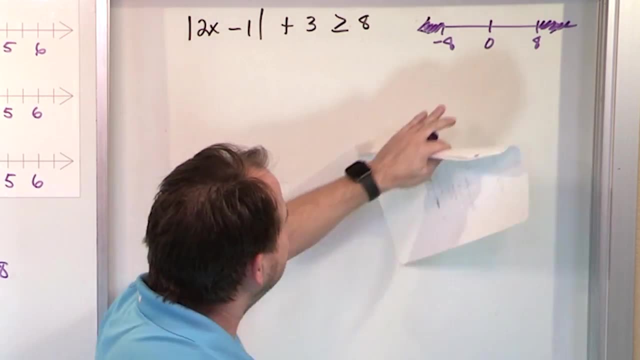 But just ignore it for now. It has to be bigger than 8 units away, So that means it's going to be way over here. This is bigger than 8 units away, and this is bigger than 8 units, bigger than eight units away, in the negative direction. So what does this look like? An and 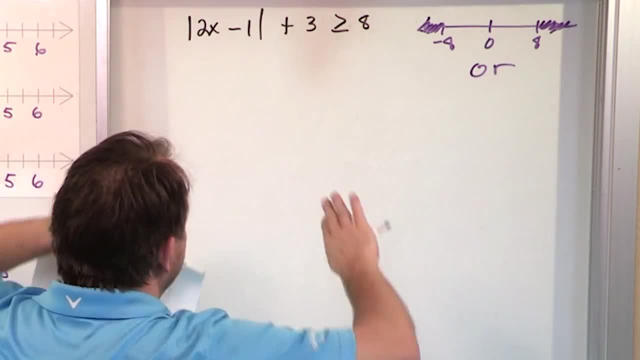 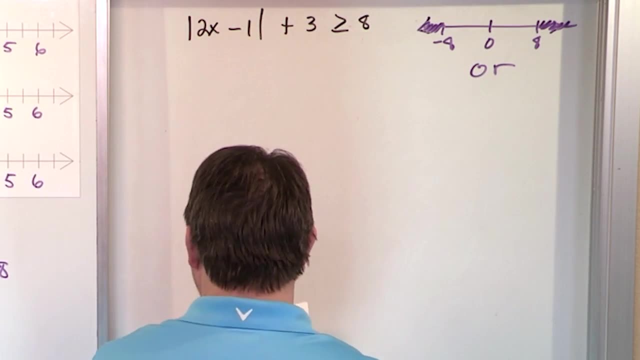 or an or It's an or, just like we've been doing all the time When it goes to plus and minus infinity. like that, it's going to be an or, And the reason I want you to know that is because the next step here is to translate this thing into that. But before we do that, we can still move. 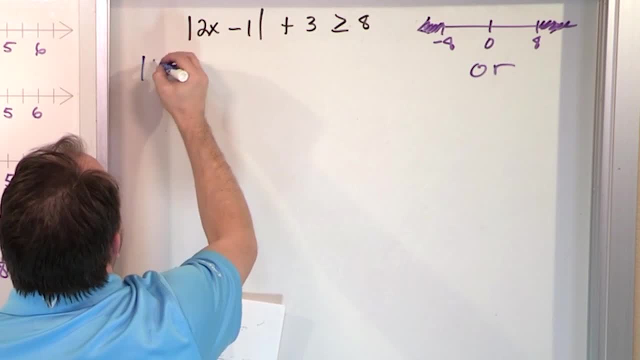 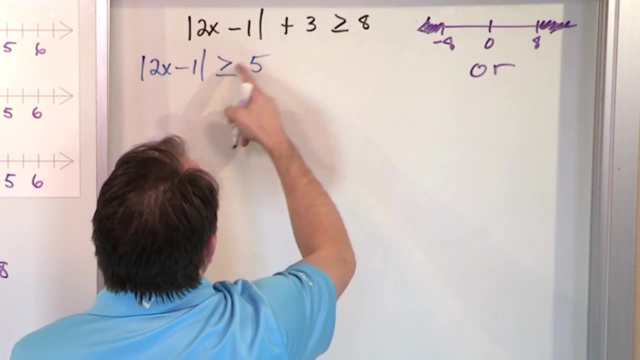 the three over and just deal with the absolute value later. So what we have is 2x minus 1 greater than or equal to subtract 3, which gives me 5.. Minus 3 here gives me 0,. minus 3 here gives. 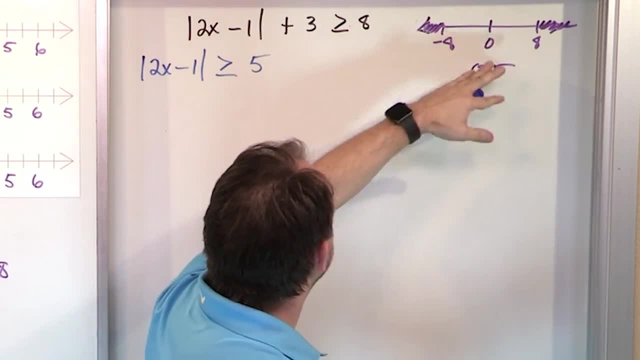 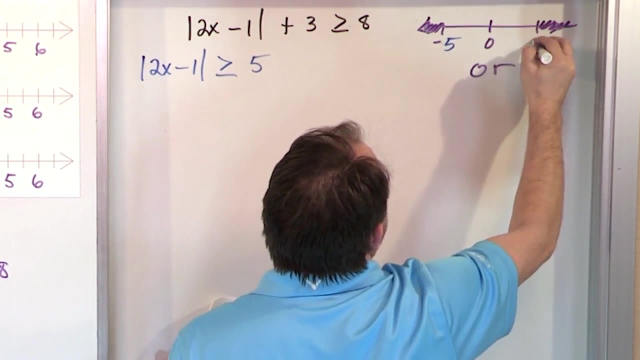 me 5.. And now I mean I could have done it another way, I could have ignored this and I could have said: just move the three over first and I can make this guy negative 5 and positive 5.. The point is, it's an or type of situation, because this is going to be greater than 5. 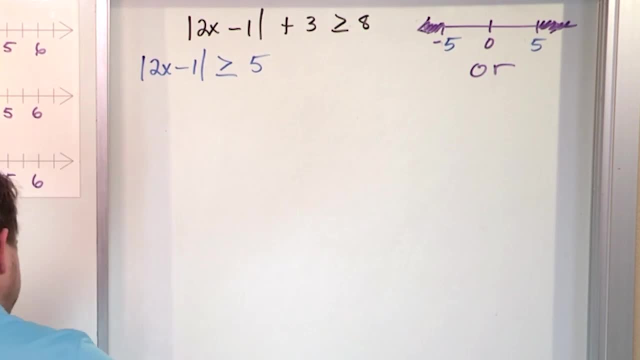 distance units away. So now we have to write the two inequalities that make that happen. It's going to be 2x minus 1.. And then we have to write the two inequalities that make that happen. It's going to be 2x minus 1. has to be greater than or equal to positive 5.. That's going to be greater than 5. 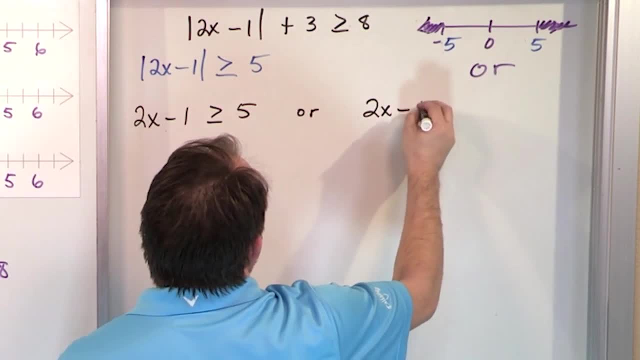 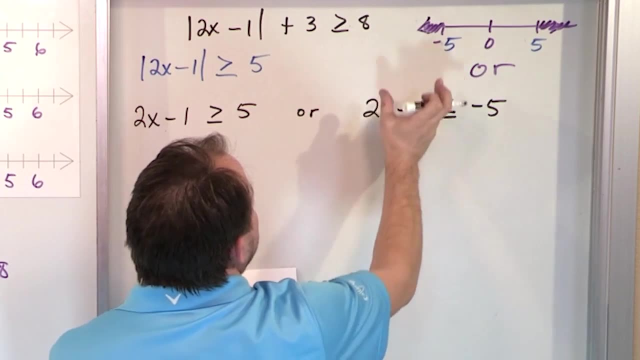 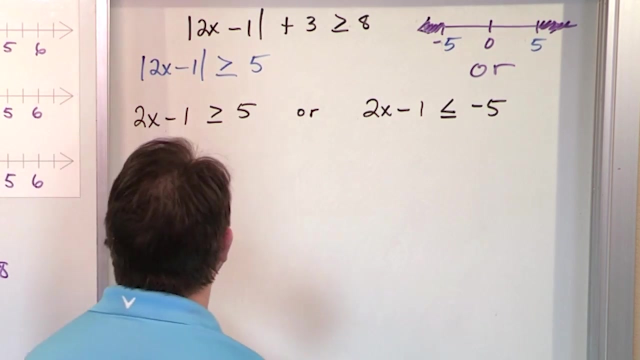 distance units over here, Or 2x minus 1, has got to be less than or equal to negative 5 to give me all the distance units in the negative direction. This quantity has to be even more negative to be farther than 5 distance units in the negative direction. OK, So now we solve both equations. 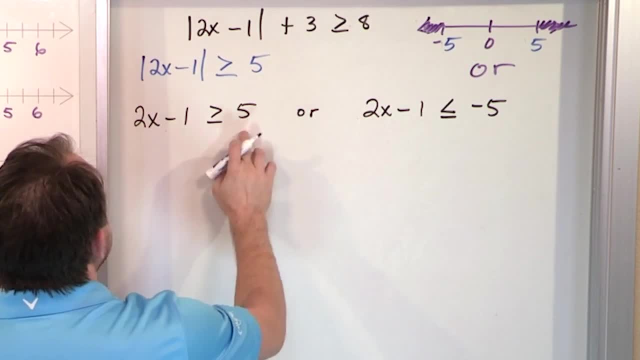 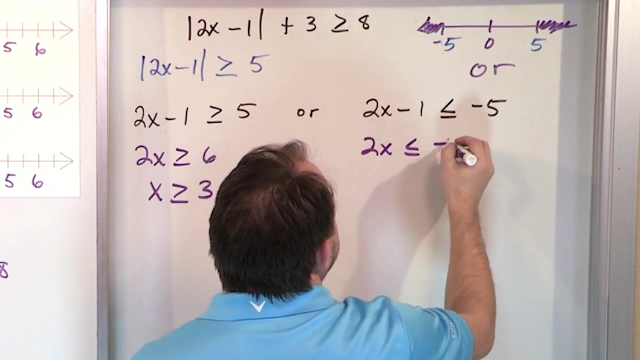 separately, or both inequalities separately. We take the 1 and move it over here By adding 1,, making 6.. And then we just divide by 2,, which gives me 3. So we have x greater than or equal to 3.. Now we do the same thing. We add 1.. When we add 1 here, we get negative 4.. And then 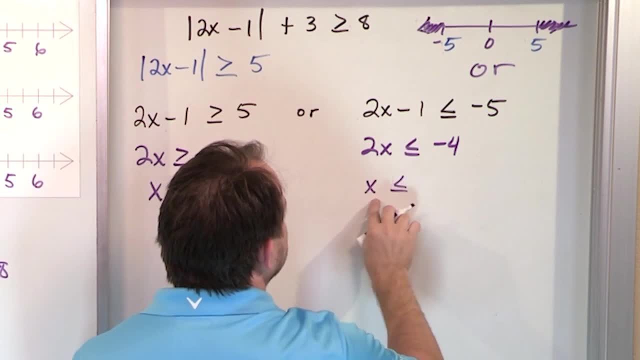 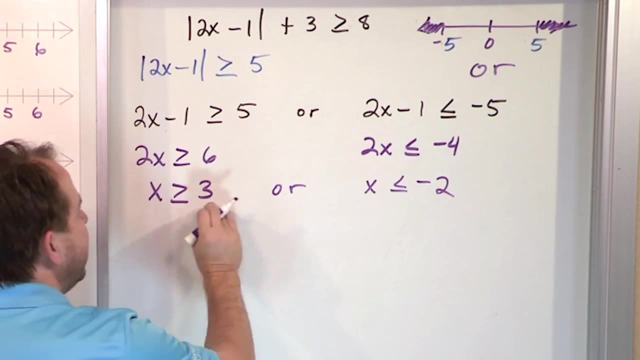 we divide by 2.. So we have x here. We divide by 2.. We get rid of it. We divide by 2.. We get negative 2 here, And these are joined by an or. So we're saying that x has to be greater than or equal to. 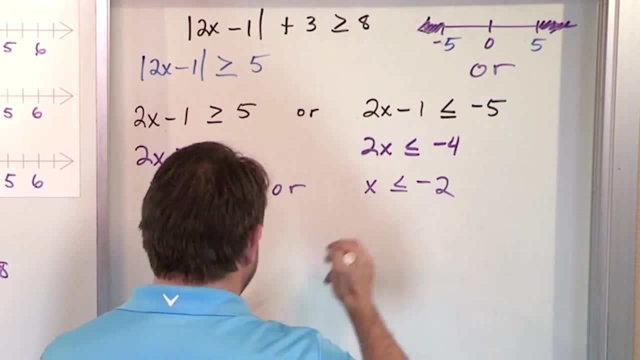 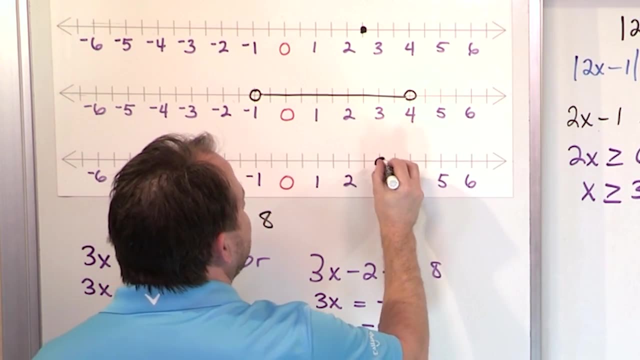 3, or x has to be less than or equal to negative 2.. So let's plot those and see what they look like. Greater than or equal to 3.. So that means a closed circle: Greater than or equal to 3, like this, Or less than or equal to negative 2.. Less than or 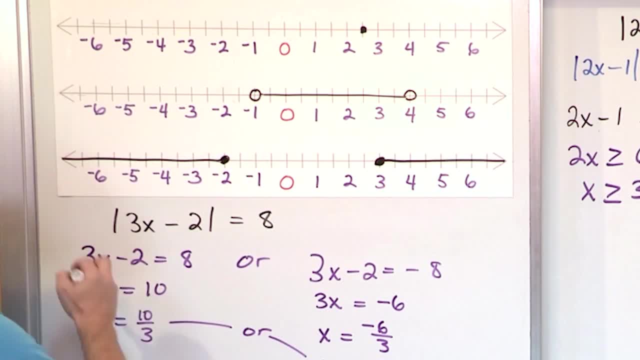 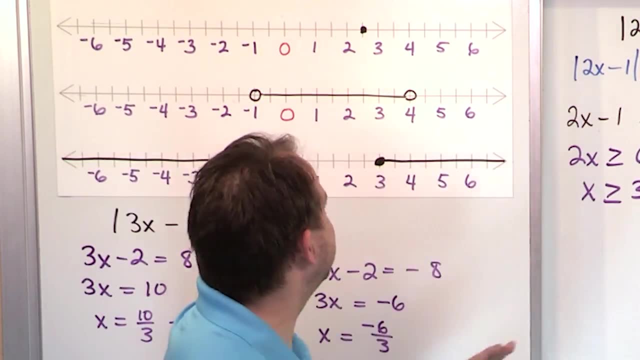 equal to negative 2.. Closed circle: Less than or equal to negative 2 means it goes this way. So what we're saying is that we have a segmented region that goes to plus infinity here, And we have a negative infinity over here which looks like an or type of situation which makes total. 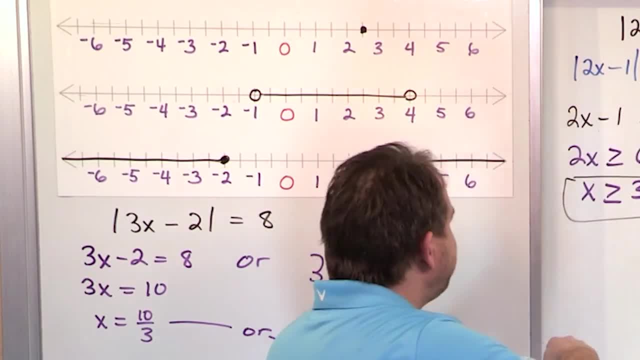 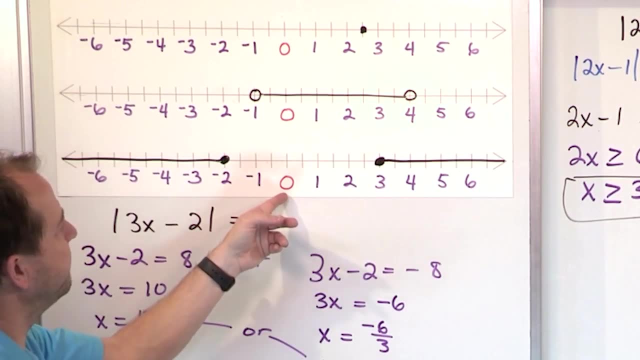 circle this guy. So which parts of the number line are out of bounds? Anything in between here is not in the solution. So let's just pick one. Let's pick 0.. Let's pick: x is equal to 0.. We're. 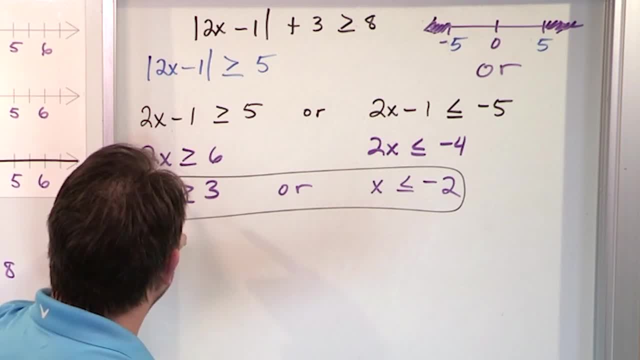 saying that it doesn't fit right. If x is equal to 0, that's not bigger than 3. And x is 0 is not less than negative 2.. So that makes sense. And if you put 0 in here 2 times 0 is 0, minus 1. So 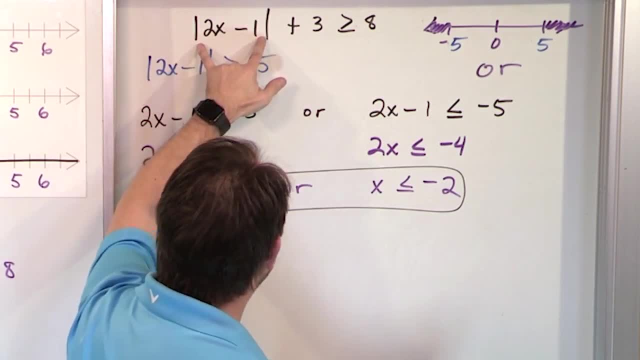 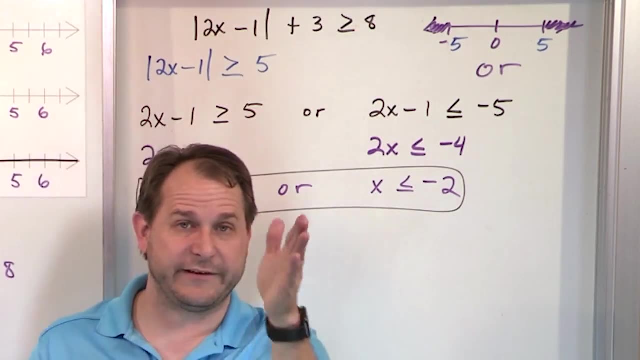 you have negative 1 inside Absolute value of that, You get positive 1.. But then you add that to 3, and you get 4.. But 4 is not greater than or equal to 8.. So that shows you that the number 0 we picked, which we don't. 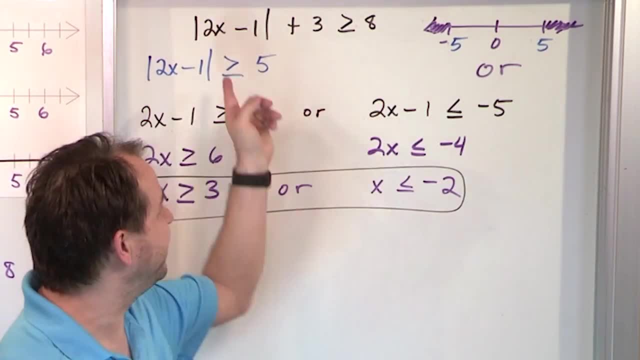 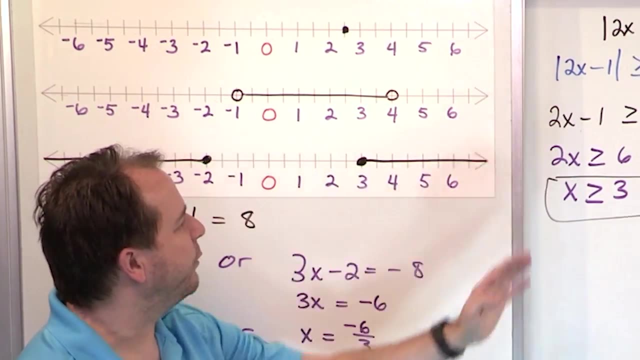 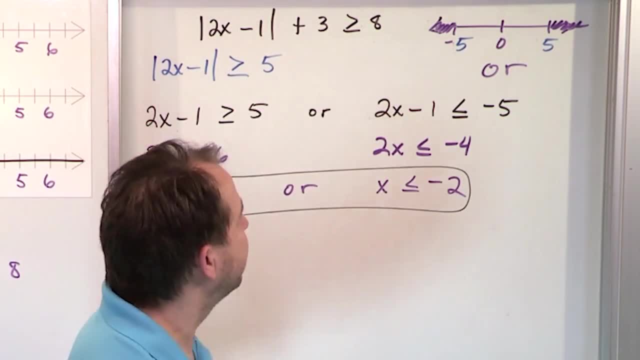 21,, 22. So that's 22. That is greater than or equal to 8. So it does satisfy it. So the way we do this guy here is we get the absolute value portion. We have to kind of know roughly what. 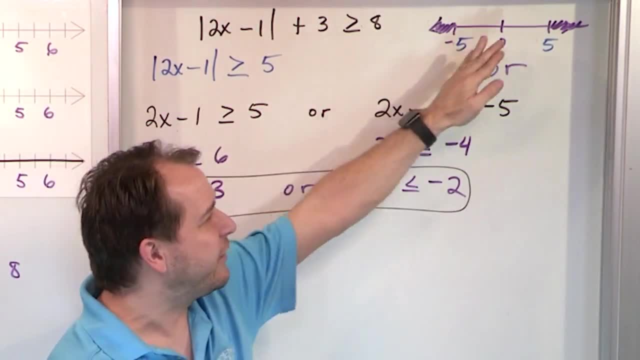 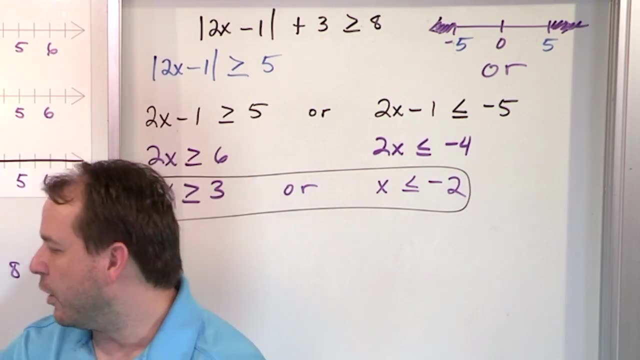 they're going to look like, to decide if they're and or or. We can make a little sketch if we want to, But we have to ultimately write two inequalities and solve them and then plot them. So we're going to get more practice with this, But it's all going to come down to for all of these problems.